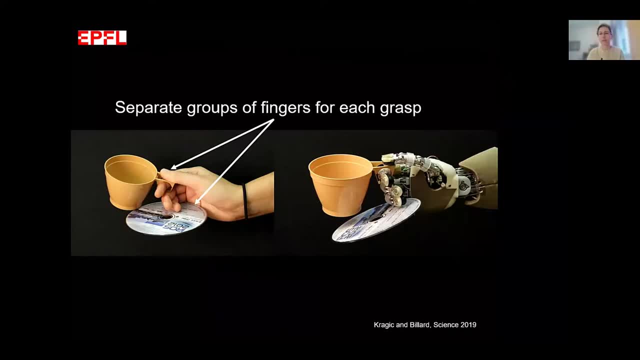 from what we see in robotics. So far, so far. we usually can pick up only one object, and at the fingertip at best. We hardly ever use the entire length of the finger, as we see here, or to pick up the object in. 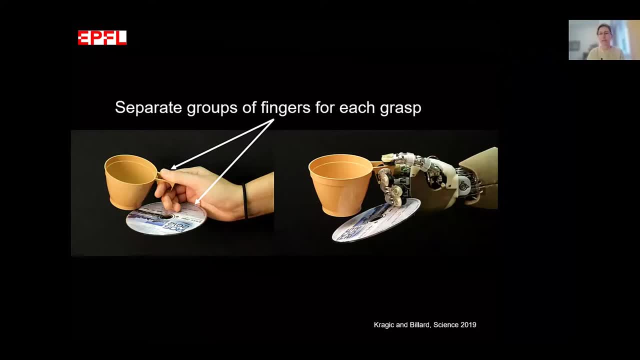 between the ring and the last finger, the pinky finger. So how can we achieve this dexterity? This was a task that we set for ourselves, that we really want to exploit this incredible dexterity that we have in human hands, Those that have 16 degrees of freedom and more, but that are barely used so far. So I'm going to 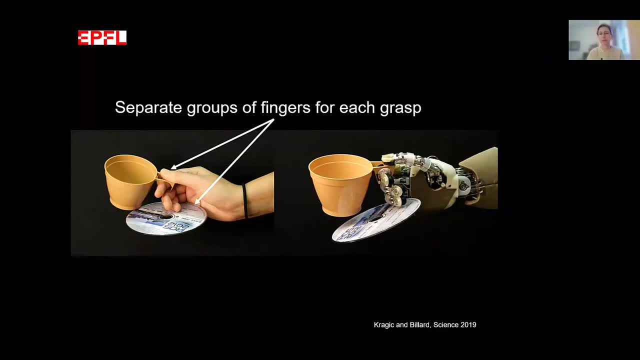 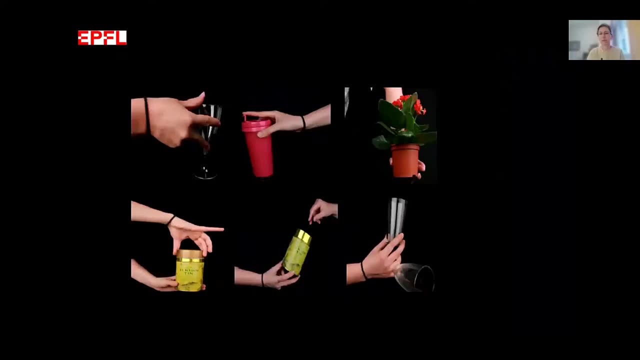 walk you through the different steps that we followed to get to this stage. So we started first by observing how humans handle objects, And there are again a very nice set of examples of the way that we manipulate daily objects. As you can see, it happens very. 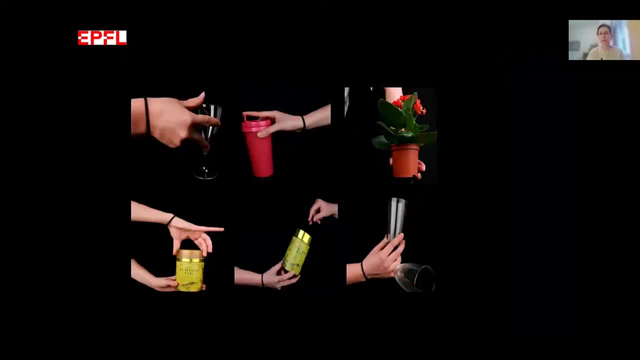 frequently that we don't put our finger just around the center of mass, as it's traditionally done In robotics. depending on what you want to do with the object, you may place your finger like in the picture in the middle. I hope you can see my mouse in the picture on the top middle. Typically, we 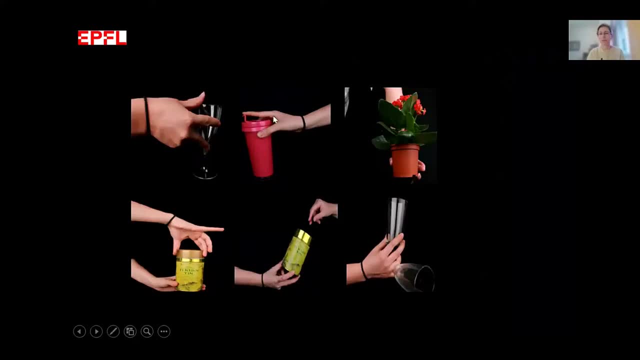 have the finger at the very top of the lead to prevent the lead from opening. This is not such a stable optimal grasp, but it's optimal with respect to the task itself, which is to ensure that the lead does not open At the bottom. what you see are examples of suboptimal grasp. 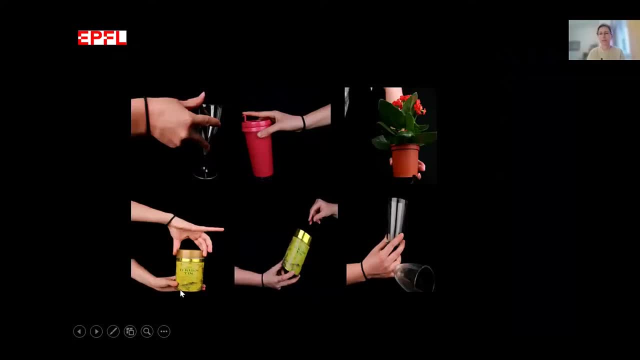 in the sense that you're not just around the center of mass, especially for the hand at the bottom of the object, on the left or in the middle, but it's optimal with respect to handing over the object to someone else. So it's been known in robotics that we place our hands on the object. 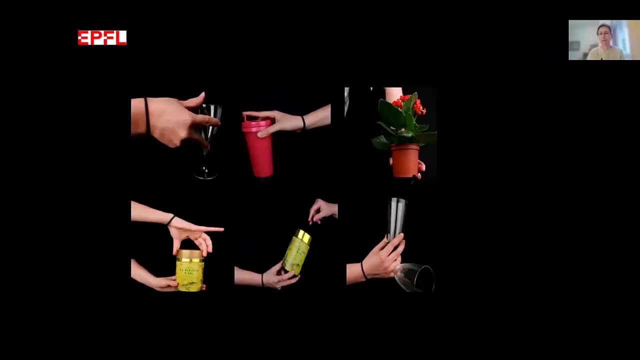 with respect to the function that we want to do on the object itself. While this is known, it's much less easy to generate those grasps and to be able to go for a particular grasp in real time in a millisecond. So our work has been twofold. One was to generate different grasps that will resemble those human. 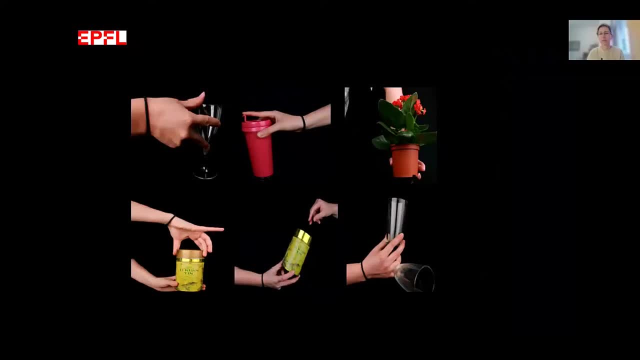 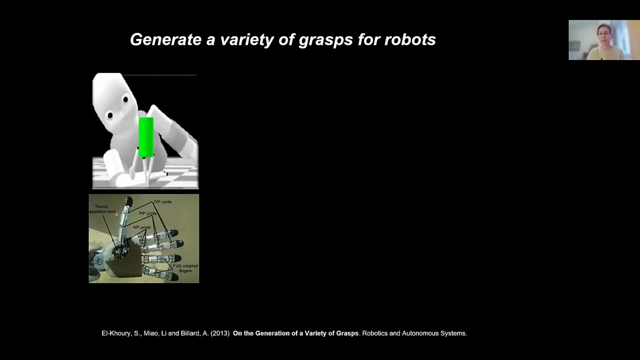 grasps and second was to be able to retrieve those very rapidly, to be able to manipulate things, as we do as humans, extremely rapidly and pick up on grasps in milliseconds. So we started off by generating a variety of grasps for our robots by doing an optimization, So we have a 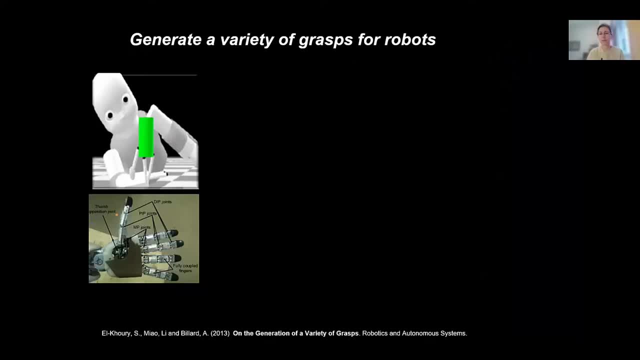 model of the kinematic of the robotic hand. Here we use the robot iCub which has the robot iCub has nine degrees of freedom in its finger And we started off in simulation We assumed that the robot could pick up just cylinder. 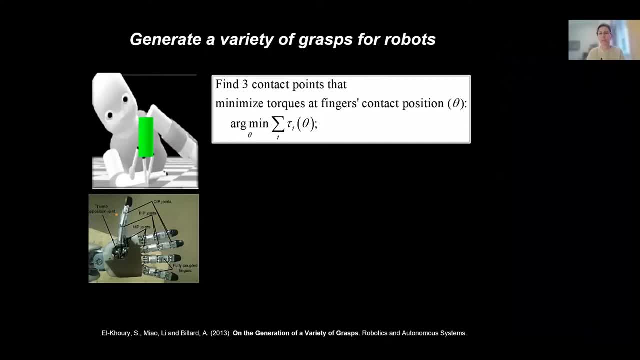 So we then task ourselves to find three contact points that will minimize the torque at the finger contact position. That's our objective function. And then we have a number of constraints. typically stability, which is force closure, kinematic stability, collision avoidance. 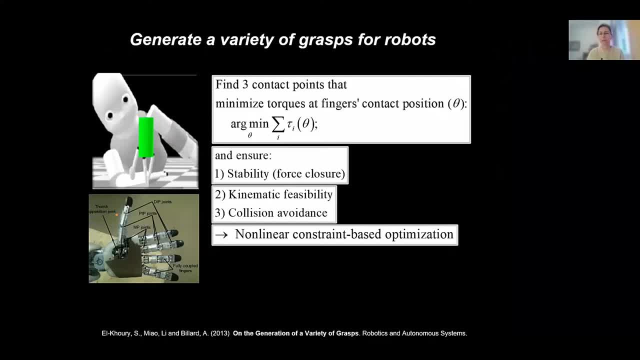 And all of this when you solve for it. it's a nonlinear, constraint-based optimization. So there are advantages to do that in optimization, Because it's a nonlinear, constraint-based optimization. you end up with a non-convex optimization and then you have lots of feasible solutions. 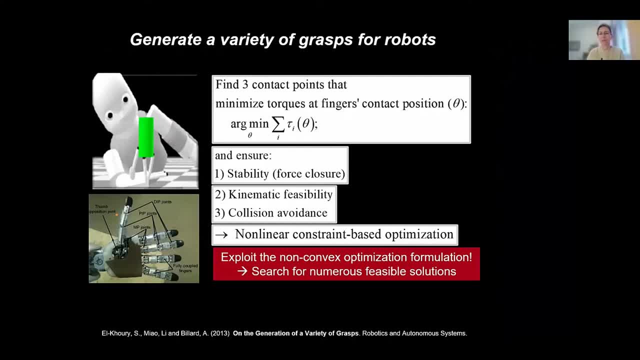 numerous of them, which you can find by initializing your solver with different seeds. And that's an advantage. Why? Because, then, we find lots of these different solutions. Here we found 1,500 of them. We then cluster them into 40.. 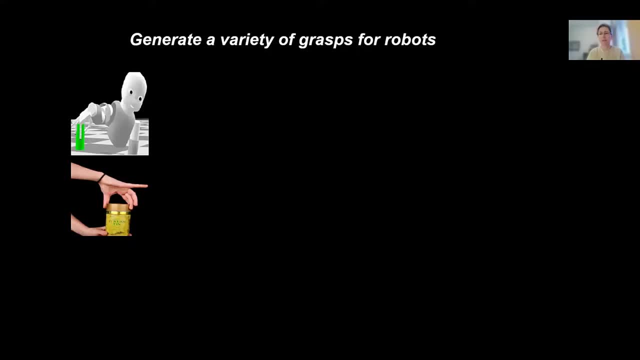 And then we did the same thing in classes, using k-means, And we found that the classes of grasp resembled those that we were looking for in the human, even though we did not prescribe the robot to have grasps that look like the human grasp. 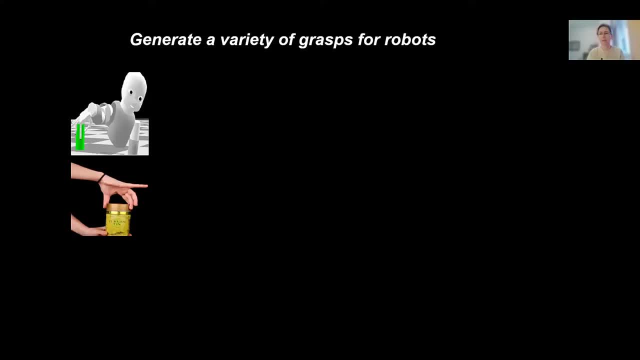 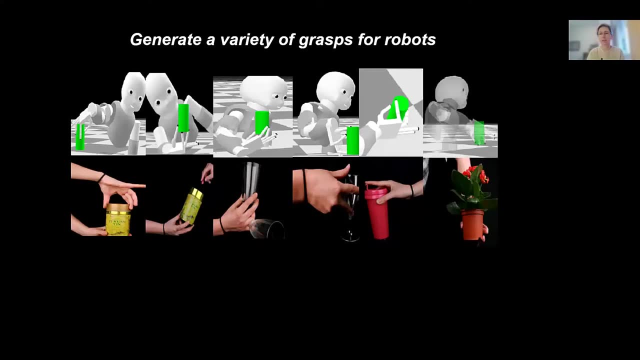 This is just out of all the feasible set of grasps on a cylinder, And observe how they resemble those different grasps that I showed you before. You see, And this is outside this notion of functionality of the grasp, It's just a set of feasible grasps. 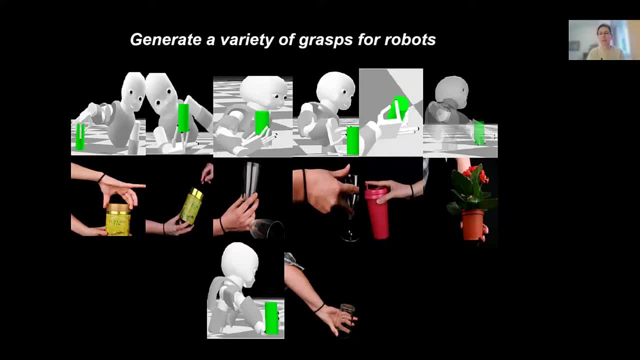 And imagine that you have this library of feasible grasps. Then you can attach those feasible grasps to different functions. Now to run this non-linear optimization takes a long time. We're already talking about minutes And in my view it's absurd to run the optimization each time you want to do a grasp. 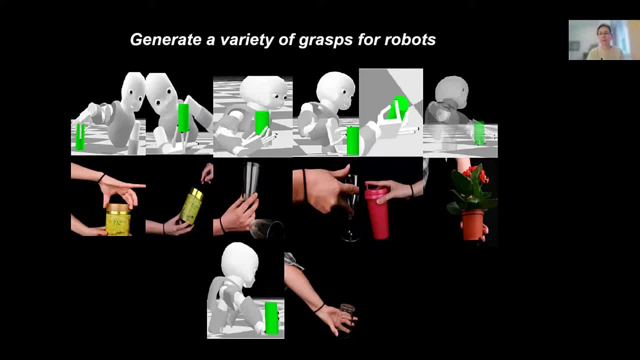 Like a human, at the beginning you learn through optimization. like a child, you learn how to grasp objects, But after a while you have learned that and you can retrieve them. So how can we go from full optimization to a non-linear optimization? 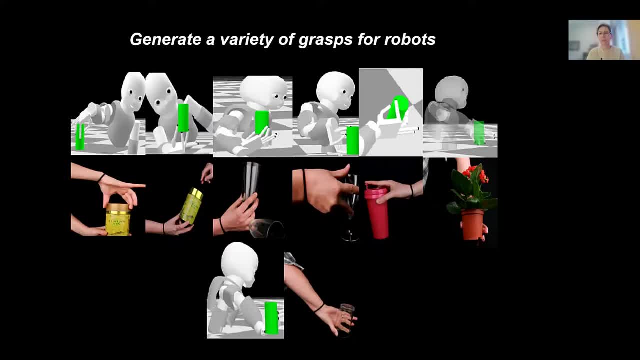 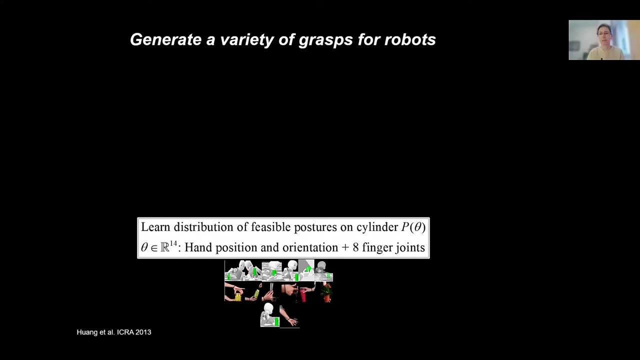 Searching for all possible feasible configuration to a learned set of those that we can retrieve in real time. Well, what we can do is that we can build now a distribution of those feasible grasps. So this distribution of feasible grasp is actually a distribution over the feasible posture on this simple cylinder. 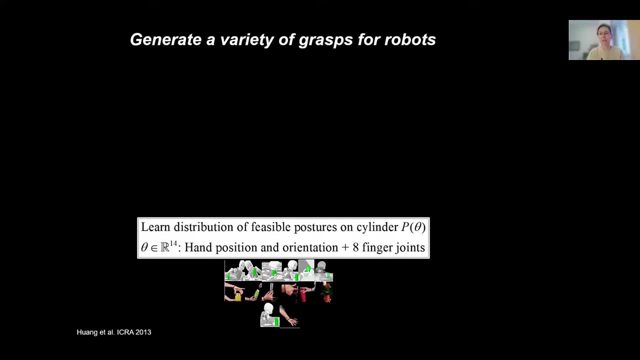 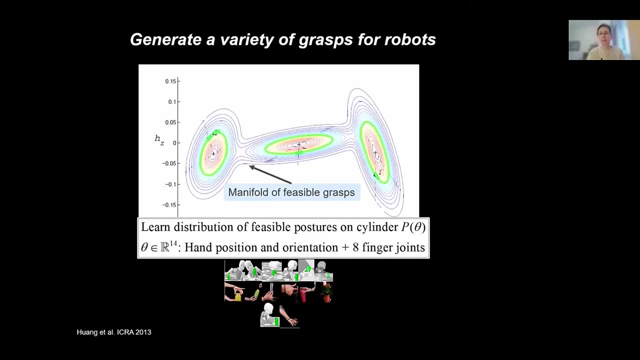 So think of it as a very high dimensional space. We have the hand position orientation, which are 14 dimensional, Plus we have all the finger joints. Now I'm showing you here is slice of this distribution, So we could learn that we did this with density based modeling in this. 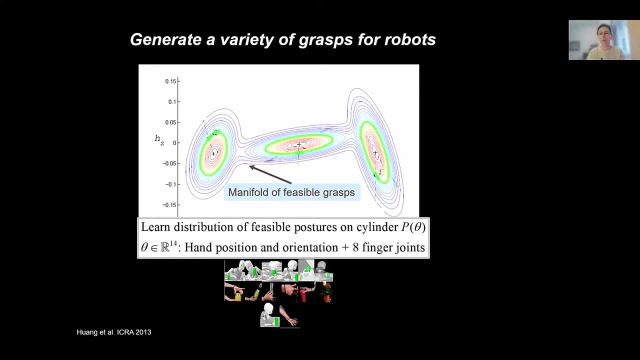 very high dimensional space, And here what I show is a cut in this high dimensional space. What you see, highlighted in these iso lines, are the manifold of feasible grasp. How do we compute this? We simply look at the likelihood of this density and those that are. 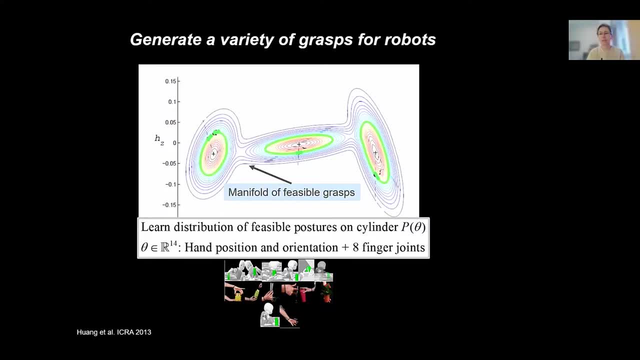 above a certain amount of likelihood and are deemed to be feasible grasps. This distribution is known in close form. That means that at runtime we can decide if we are in the infeasible grasping region or the feasible grasping region. 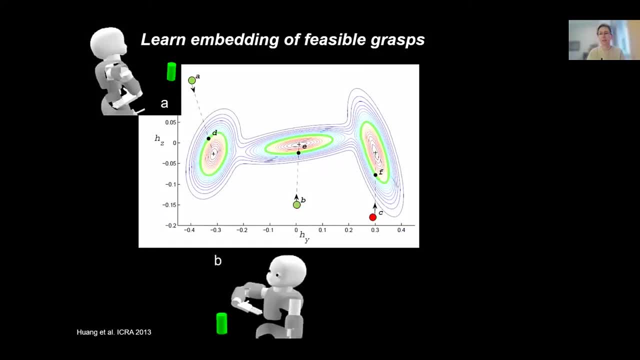 Now assume that you start somewhere in the infeasible space which is typically before you actually grasp the object. You're far from the object. Then, because you have this distribution in close form, what you can do is a simple line search. This is super quick. 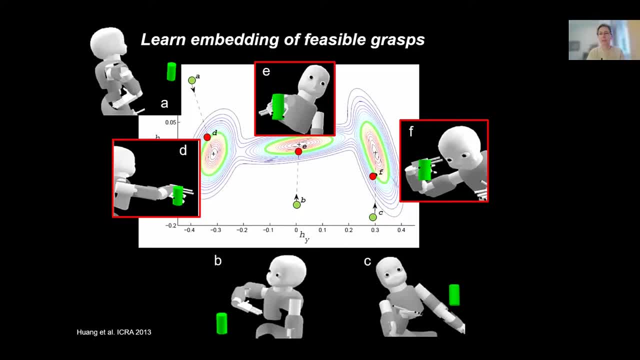 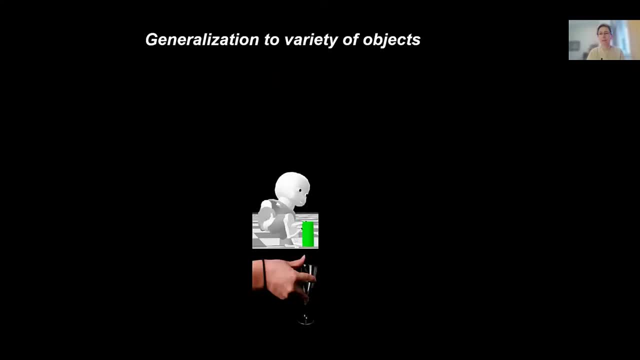 You can compute that in millions. You can do this and pick up the closest, grasp, the closest to your joint configuration space. So observe how we can use that now. It was a real robot, So I'll show you here a couple of examples. 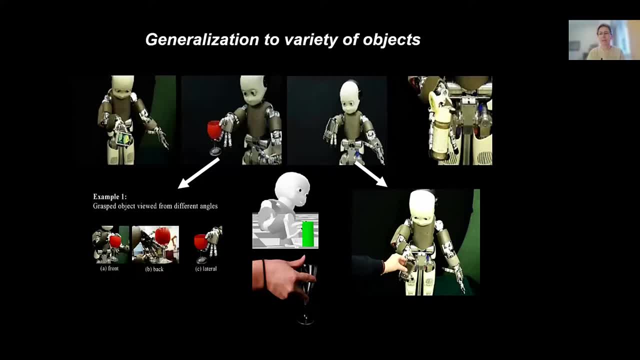 You'll be surprised to see that we are using here a different object than the cylinder, And that's the beauty of it is that you can train this on a very simple representation of the cylinder. This generates this feasible grasp, which are pre-shapes, if you want. 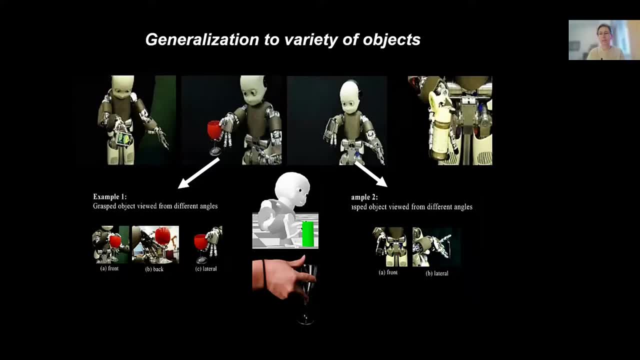 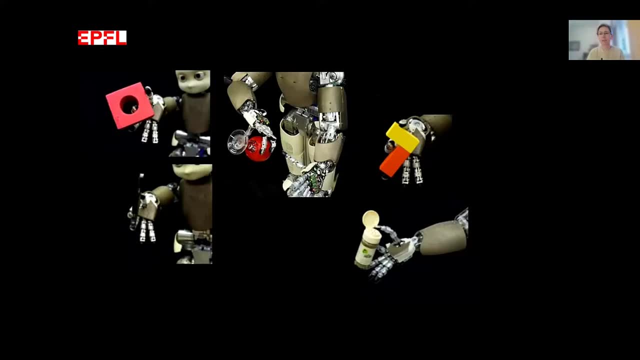 And once you use this pre-shape and you close on the object, you find out that you can close on many different objects. I'll show you other example here for another set of feasible grasp that we've seen before with this pre-shape. 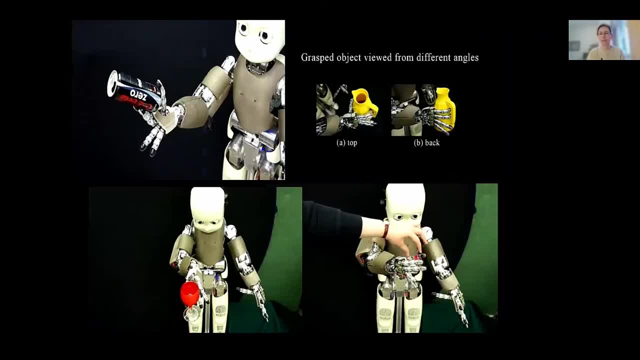 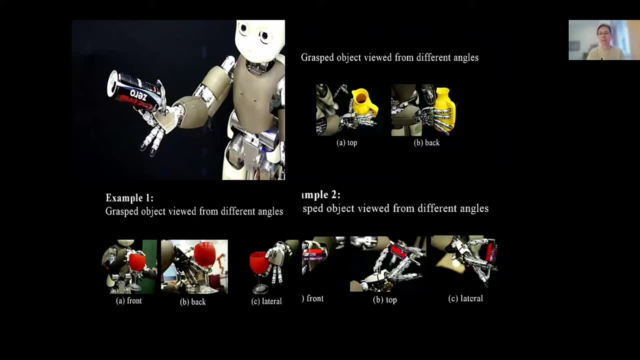 And now we can use those to close, as you can see here on a very complex object with a nice positioning. I partly like the example on the bottom right Here. observe that you have the two fingers that are side-by-side and the two fingers that are side-by-side. 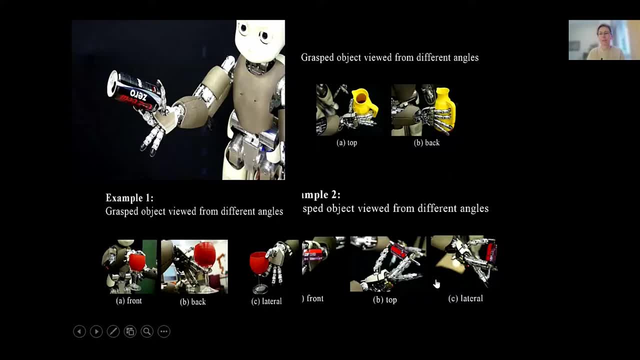 And the two fingers that are side-by-side are connected to the pin of the object here as a screwdriver, And this is becoming one step closer to the very first image that I showed you, which is to be able to pick up object by using the entire length of the finger. 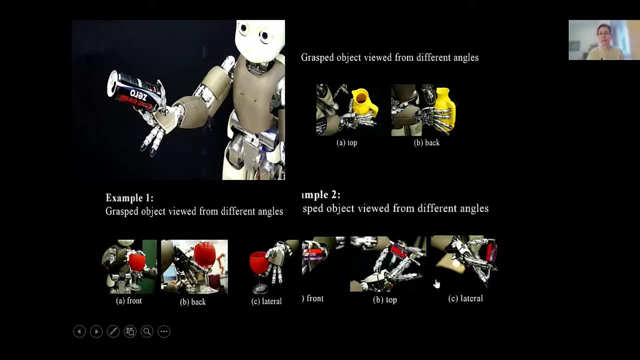 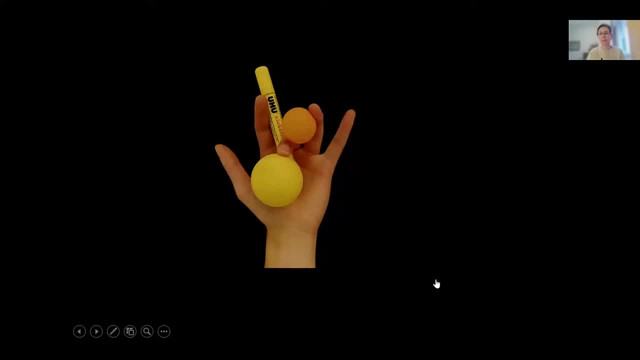 So this was a very first step that we did towards this idea of exploiting the entire dexterity of the hand. Now I'm going to present to you most recent work in this slide. As I said before, one thing that is absolutely amazing is the fact that humans can hold many objects in the hand. 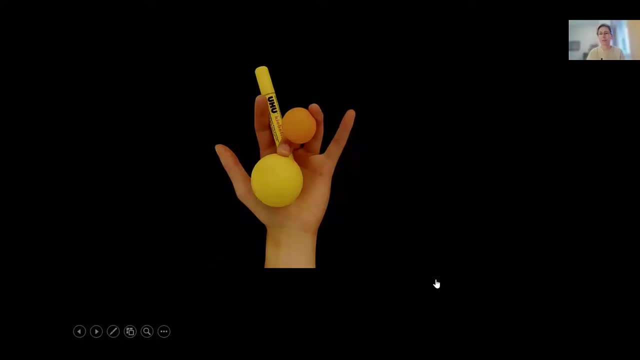 And this is the typical example of this dexterity. What is difficult is not just to hold the object stably by combining the fingers, but also to make sure that the object will not intersect with one another. So you have to place them smartly in such a way. 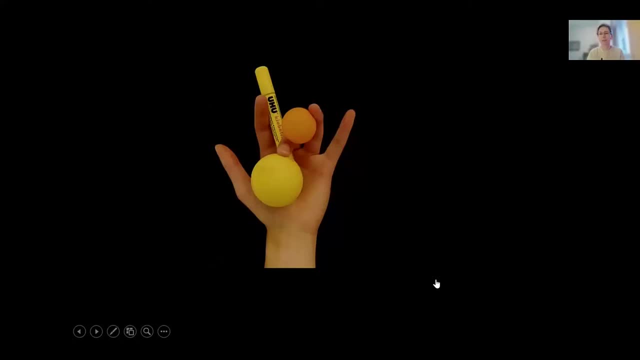 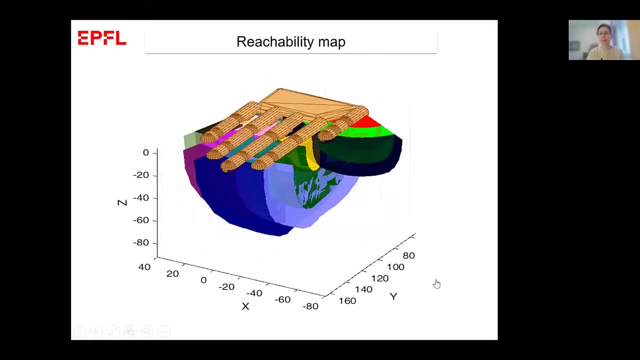 And if you wanted to pick them, then you'll have to pick them in a certain ordering to be able to place them in the hand. So how can we approach this? Well, we started off first by saying we need to have a representation of what is reachable by each of our fingers. 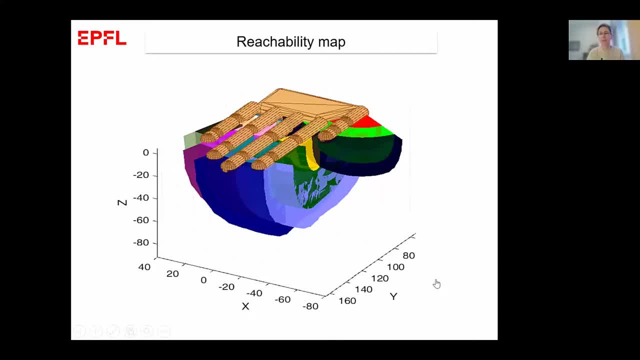 So we need to have a model of this reachability map which are represented here. So we go finger by finger. We have the kinematic of the hands, So it's easy to do that. in simulation We can build the sums workspace. 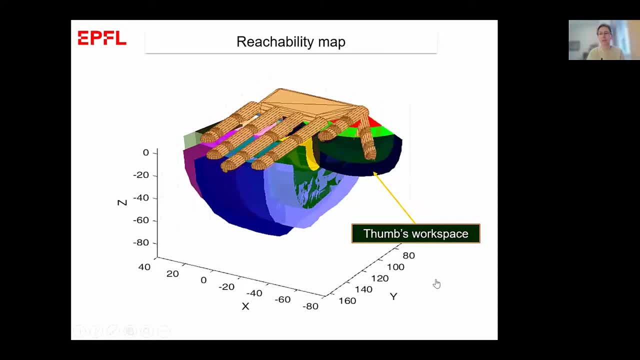 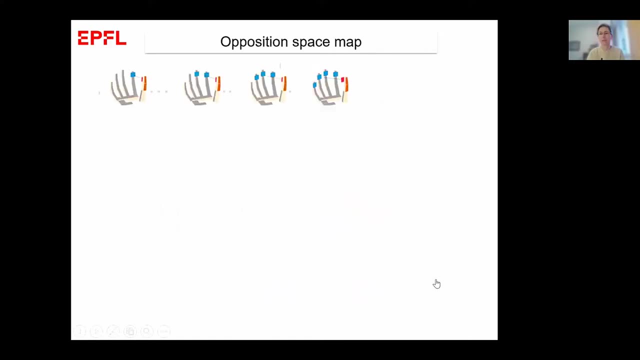 typically by sampling or the position of the sum. We can do the same for the index, the middle finger and so forth, And now we can represent this in close form, similar to the density-based estimate that I presented before. Second is that we need then to find how we can pick up object with our finger. 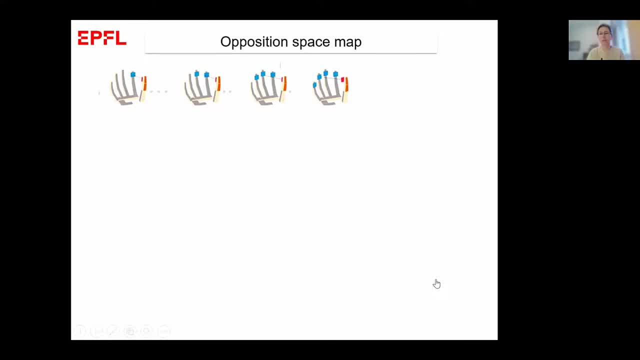 And we revolved here to a concept that had been developed in human motion science, which is the notion of opposition space. Now opposition space have often been studied in terms of just the finger opposing the index middle finger, etc. Now we push this further. 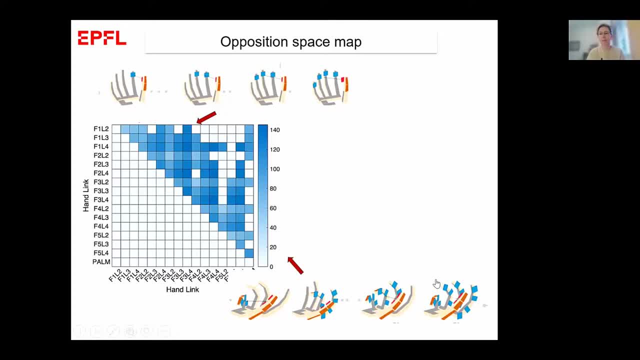 to say: well, we want to have the opposition space over all possible fingers, And that's what you see here, And I know it's difficult to look at this map. So just take it as a representation, as a vague representation, that each of those entries represents now pairwise opposition across each of the phalanxes. 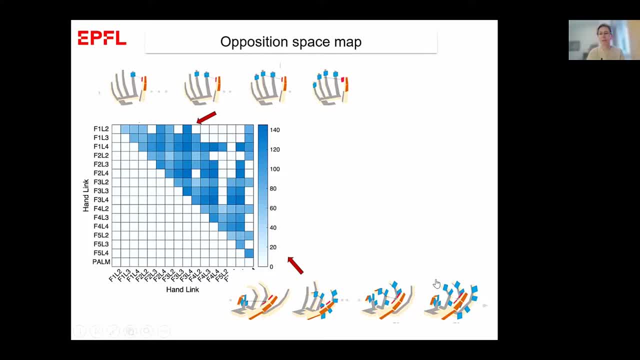 And so you see that we go from the very trivial one, which is sum and index, to go and have opposition between the middle finger, ring finger and so forth. Now, once we have this, we need also to compute this self-collision map in Cartesian space. 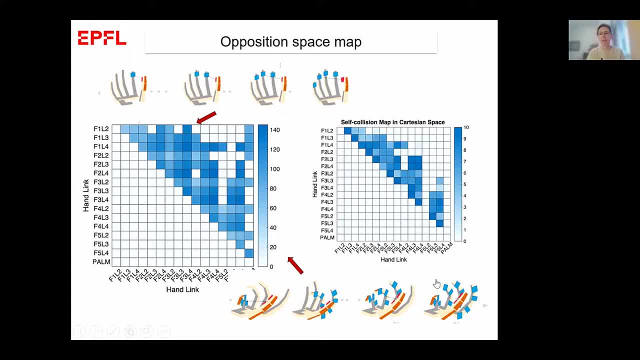 to make sure that when we compute a motion for each of our fingers, they do not self-collide with one another, And we need to also have a representation that this workspace may shrink as I start moving some of the fingers. So how do a pair of oppositions reduce the workspace of the other finger? 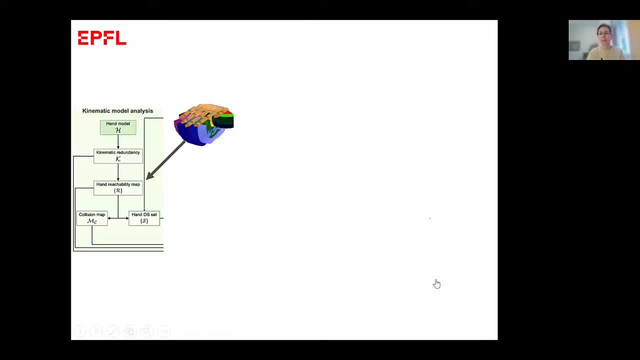 I will not go through all the details of how we are solving this, but I'm going to give you a brief overview of the optimization process. So again, we revolve here to full optimization first. So we have this kinematic model of the hand and the workspace. 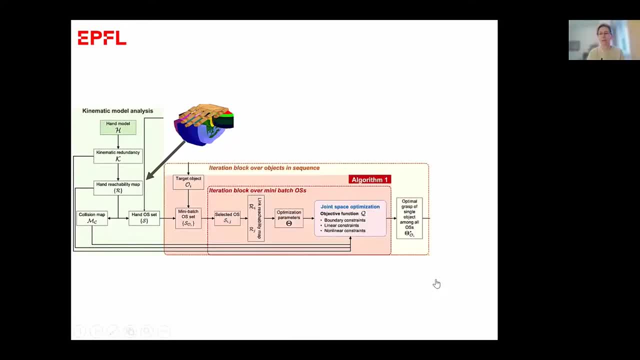 So we start with this, this hand reachability map. With this, then, what we need to build is an algorithm that allows us to search for something that is reachable for our robotic hands, because the model that we have is for the human. Now we have also the kinematic of the robotic hand. 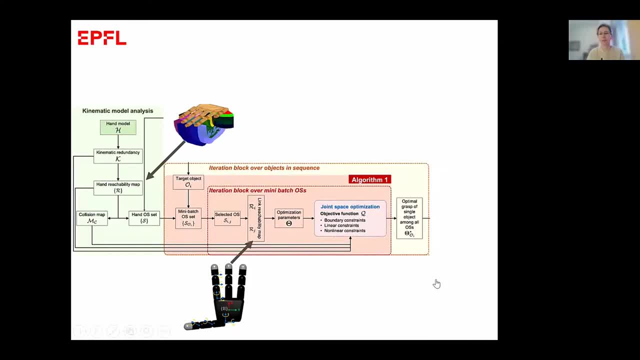 We have a notion of this opposition space in the human hand, which we can then map to the opposition space in the robotic hand And then, finally, we can solve, as a constraint optimization space, a constraint optimization problem in joint space, similar to what I described at the very beginning of the talk. 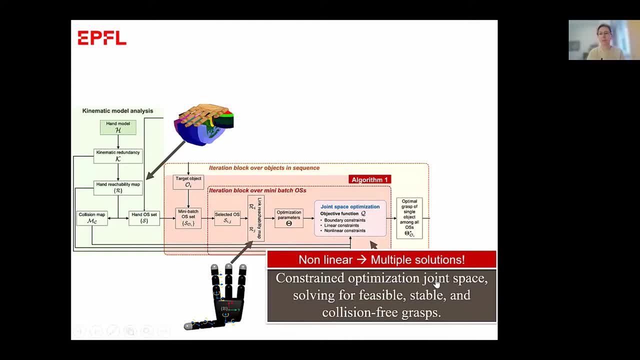 solving for feasible, stable and force closure grasp and also collision-free grasp. But now observe that what we are doing is not just for one single grasp with three contact points, but we are looking for all possible oppositions of the figure that will allow us to pick up objects. 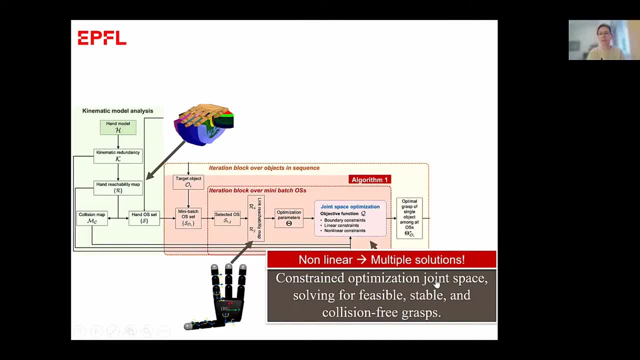 This is again a nonlinear optimization problem, so it gives us multiple solutions, And that's the good part of it. Similar to what I said before, this multiple solution will allow us then to choose among many different possible solutions to pick up the object in the right order. 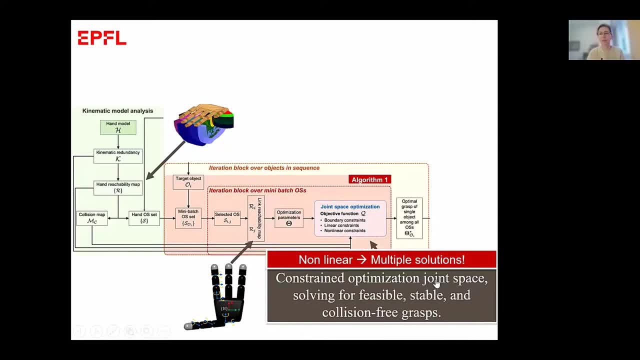 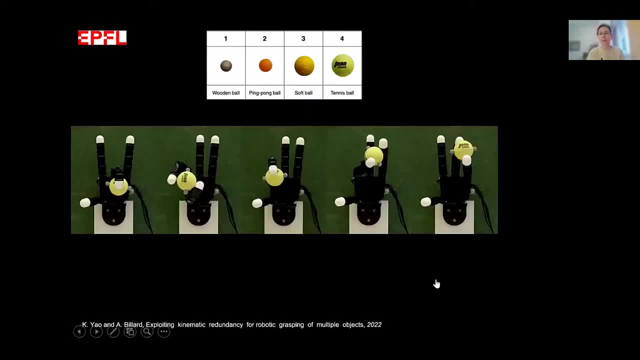 So let's just stop now at this notion of using this opposition space to find all possible ways in which we can grasp objects. I'll show you a couple of examples of how we can do that. Here is an example of this. Here you have five different examples. 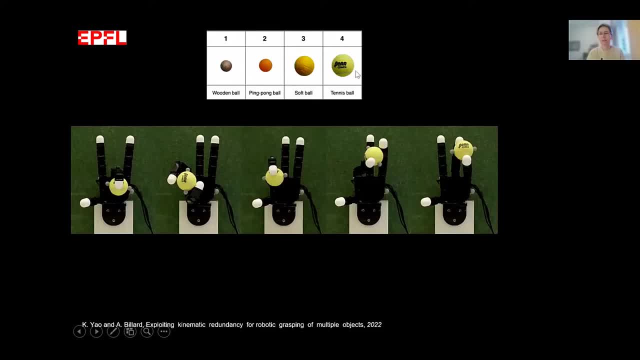 of how we can pick up the large ball, the tennis ball that I show here on top on the right-hand side. Observe how we can recruit, sometimes two fingers, sometimes three fingers. Observe that these are not just the thumb and the index. 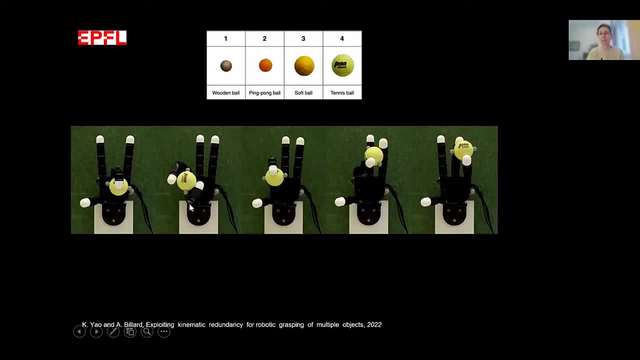 Typically, aside from one example, the second one from the left- all the others are using either the last fingers or just one single finger on the first one. Very interesting grasp. Some of them leave a lot of room for picking other objects, as you can observe. 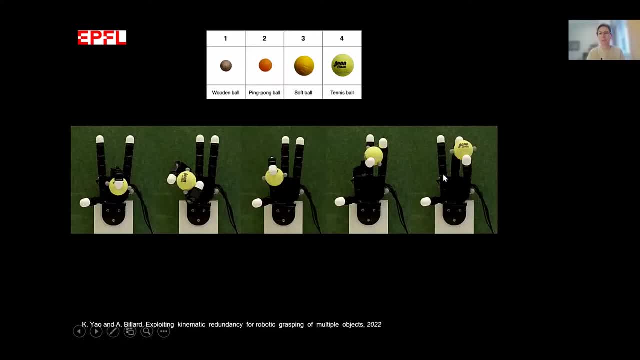 typically for the last one, and that leaves still the thumb and index free. So these are interesting grasps that we can reuse, and I'll show you how we can do that. Now. that's the solution for the large ball. Now, if we change the size of the ball, 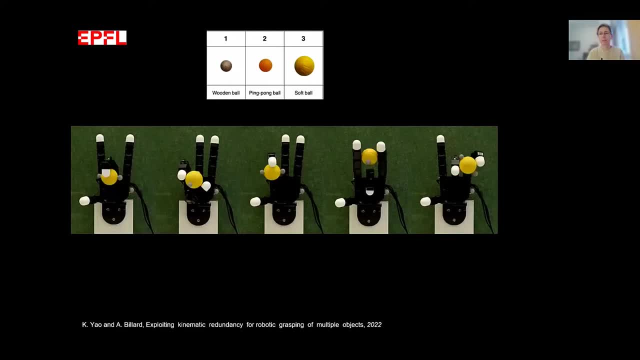 and we go for this soft ball, the orange one, we see that we end up with a different set of grasps because of course we have to balance both the position, the size of the object and the aperture of the pair of oppositions. 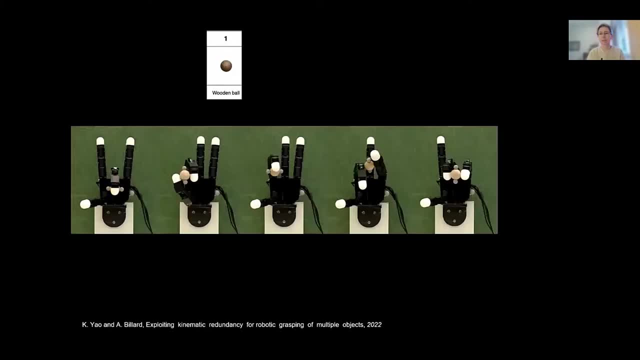 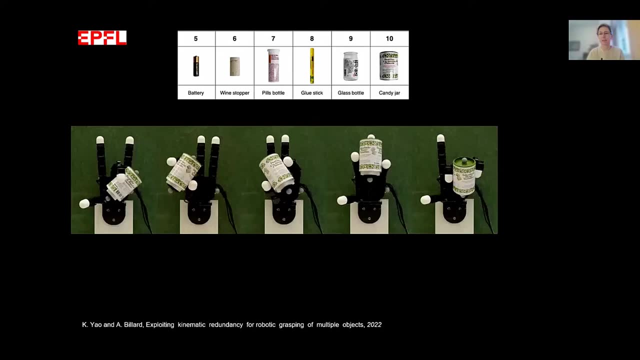 We go down with other balls, we see different types of grasps and so forth. We can do the same type of computation for other objects, typically cylinders. Here we start with a large cylinder and then we go our way through other cylinders. 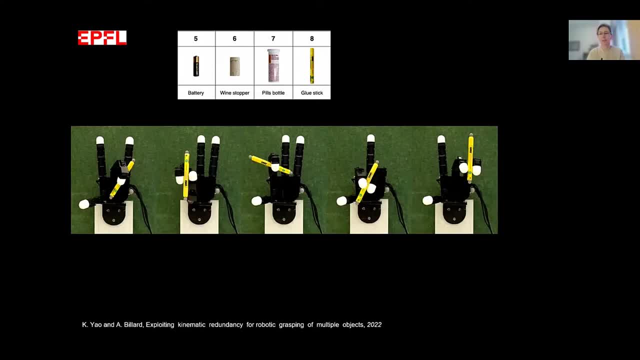 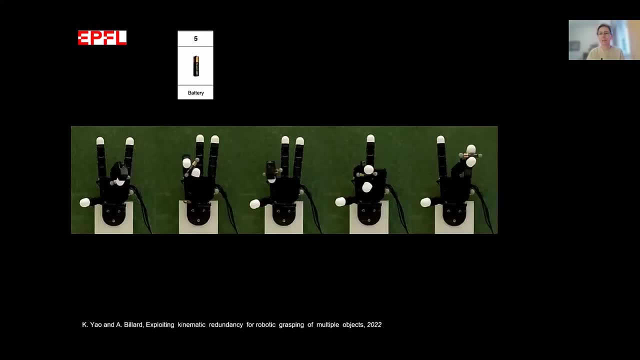 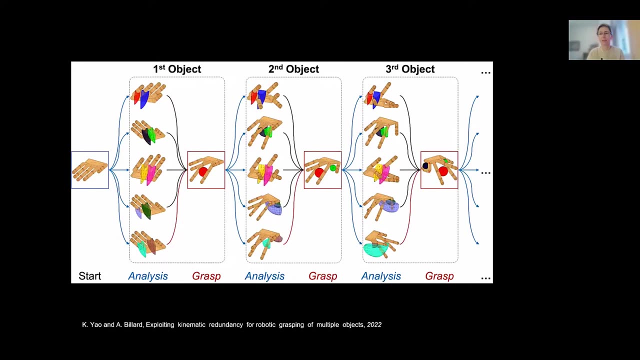 smaller. here is a typical cylinder that we resemble a pen, and we can go down with an even smaller cylinder and so forth with a tiny one. Now, this library of grasps allows us now to tackle the problem that I told you at the very beginning. 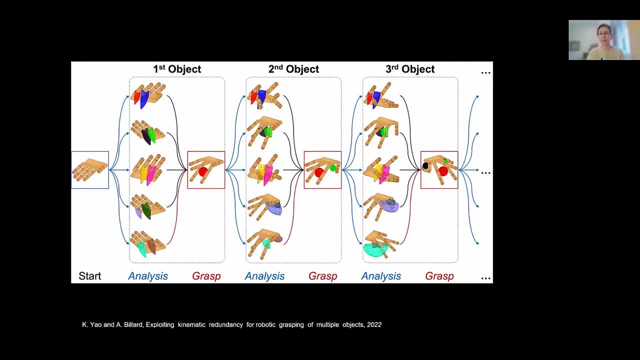 How can I place different objects in my hand? And the way we do it is iteratively. This is illustrated in this figure. We start by analyzing. I give you a first object. How can I pick it up? What are the range of opposition space that I can use? 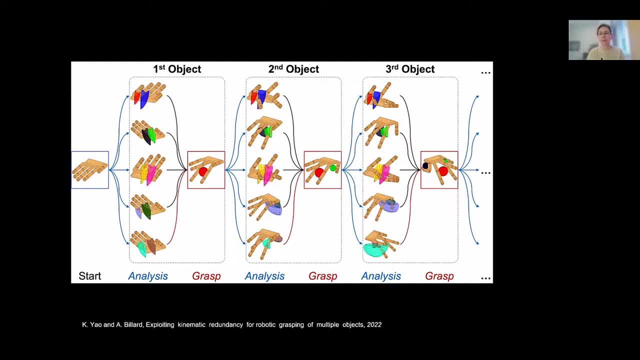 the range of grasps that I can use And then, once I have picked one that you will use, the least amount of contact points, of course, because I want three, many different points. then I can pick up the second object that we see in the middle here. 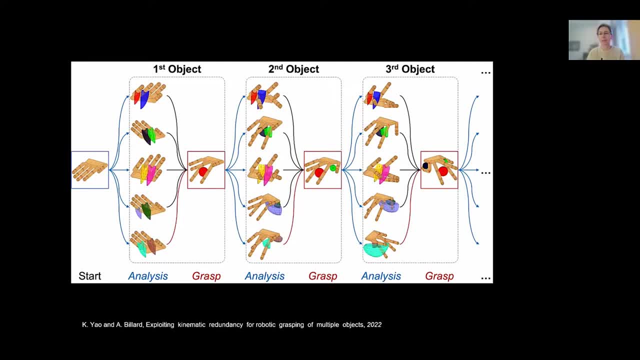 the little ball and then, finally, I can pick up the third object. So at the minute we can pick up three objects, but the entire pipeline could work, of course, for more objects if we had more degrees of freedom. So how does the pipeline work? 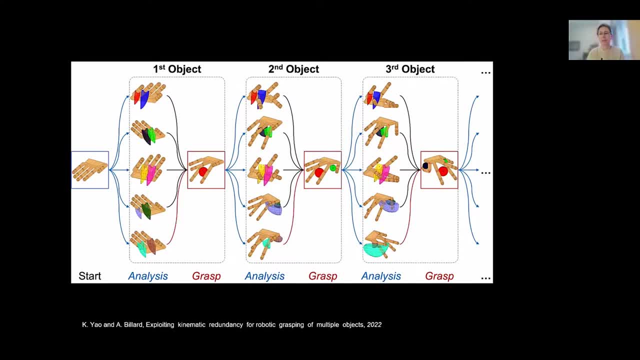 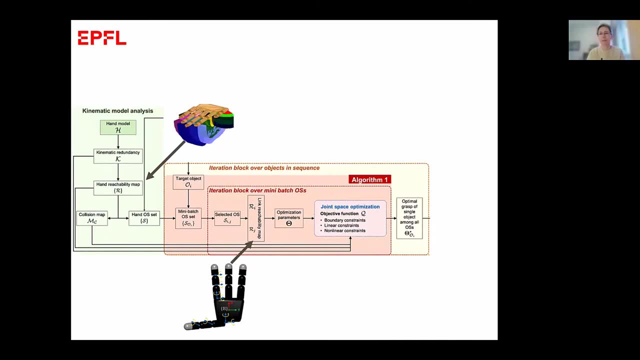 We go back to the schematic that I had before. So we have this: this is the first object, and this is the second object, and this is the third object, and this is the fourth object, and we just analyze this for one single object. 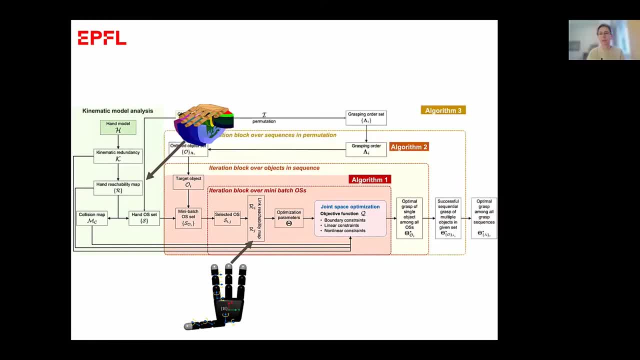 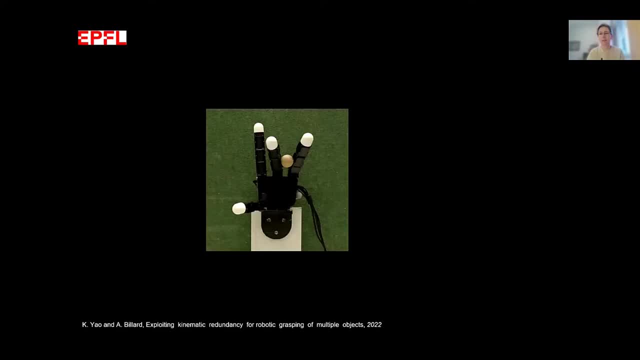 and then we repeat this for second object, third object and so forth. So I'll show you here examples of grasps that we've seen before and we can use them in sequence. We start by picking up the small ball that we've seen before. 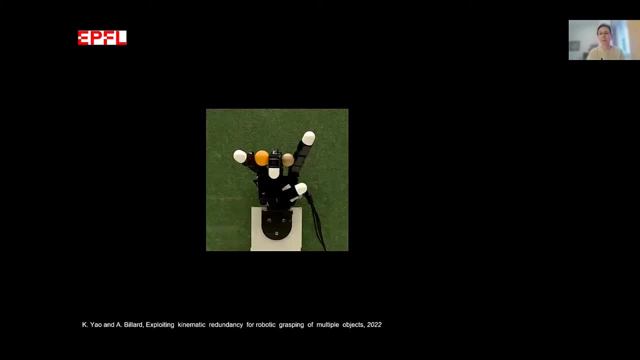 we can then use the other two fingers to pick up the second ball, and now we use just the thumb to pick up the small cylinder. We can do this also for a larger ball with a cylinder in the middle and then a large cylinder with the thumb and index. 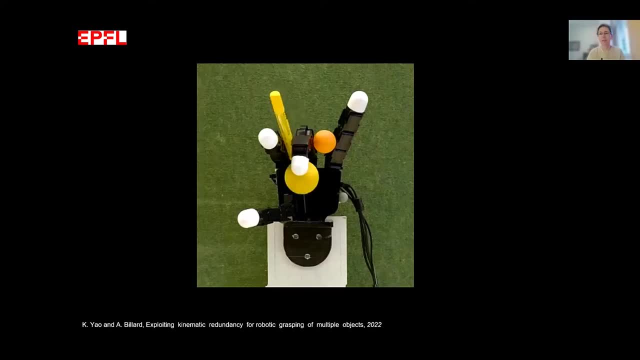 And finally this one which we've seen at the very beginning of the presentation. So that, to me, is a major change with the way that we pick up objects in robotics traditionally. It's really at last using, as I said in the introduction. 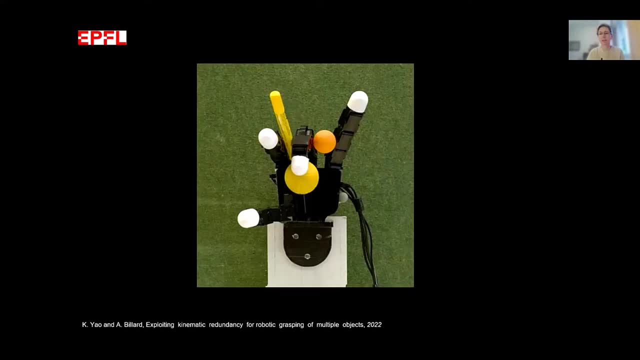 this entire dexterity that we've painfully put in these beautiful hands, the Allegro hand, which is 16 degrees of freedom, which I really find as an extraordinary hand. Not only is it very fast. I haven't shown any example of fast control. 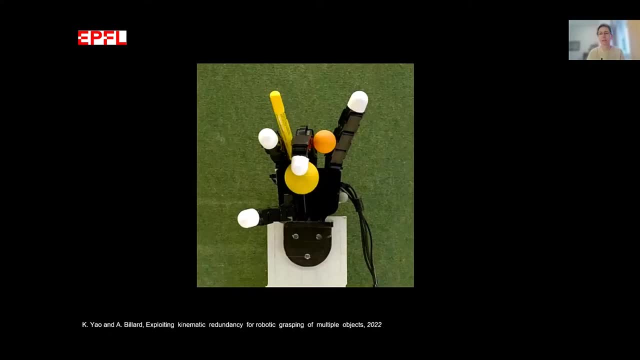 but I'll show at the very end of the talk how we can do that. But also it's very dexterous and there are many degrees of freedom- 16 of them that we can use- POIs. So I'm very happy with this result. 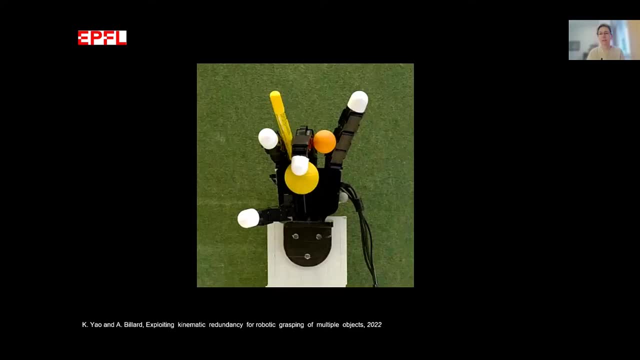 and I hope you can share some of my enthusiasm With this. I'd like to go one step further. Oh yeah, I forgot the fourth object, which we managed to also pick up, which is one more example of going even beyond some of the human dexterity. 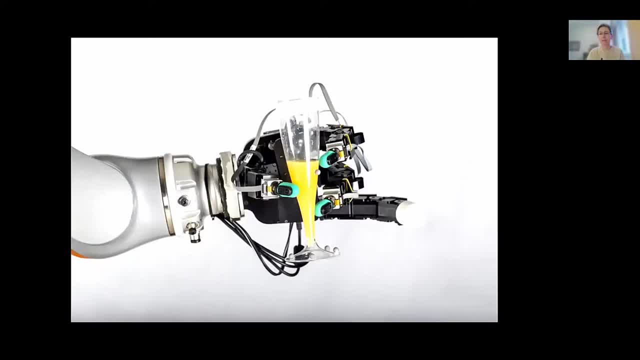 Now one step further. Of course, when we pick up objects, it's not just to hold them in the hands statically, as I've shown, but it's to manipulate them, And I haven't said anything about controlling the object in the hands so far. 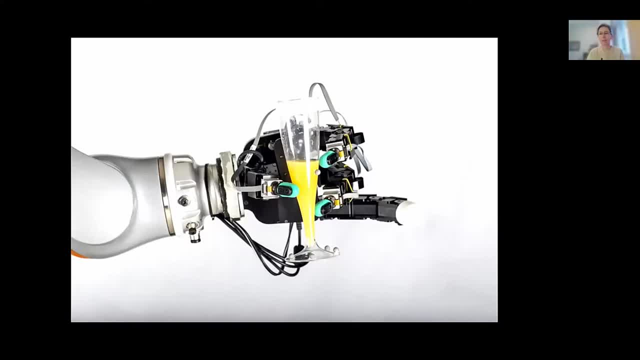 I was only talking about placing the object in the hands such that you could stably hold them, but we are not manipulating them. As you know, usually when you pick up objects, you actually then will move around your hand, and so that means that the object 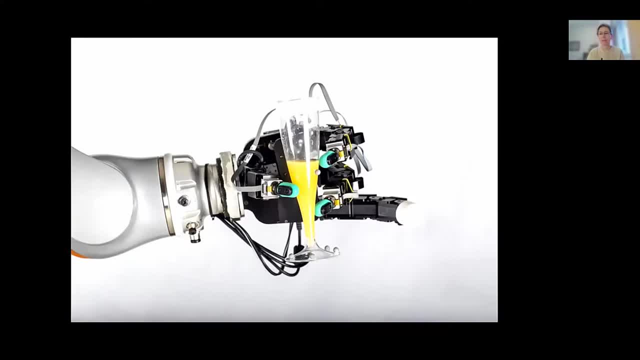 will move around with you and you will have to make sure that the object will not drop. When the objects are made of a single material, then it's usually not too difficult to hold them in the hands, unless their mass distribution is inhomogeneous. 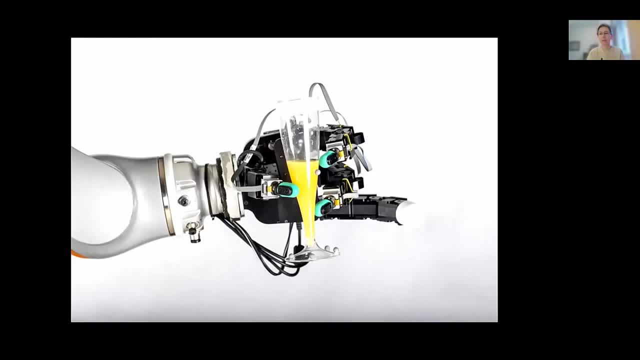 as is the case with typically these glasses. If you move around this glass, what will happen is that the contents will start floating through the glass and hence the moment of inertia will start changing and you'll have to counterbalance force. I haven't said anything about force control. 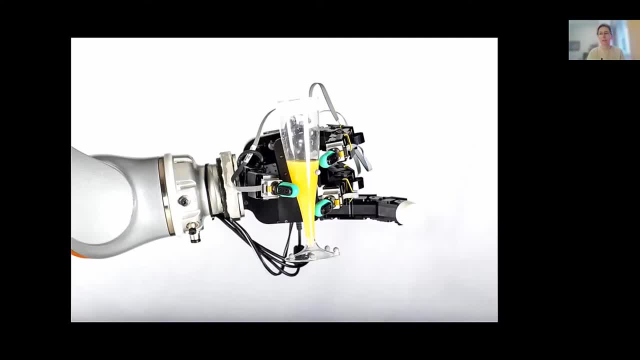 but it's obvious that force control has to come up here. Until now I was talking only about kinematic control. Now we need to do force-to-control, and to do that, of course, we need to measure force, which we can do. 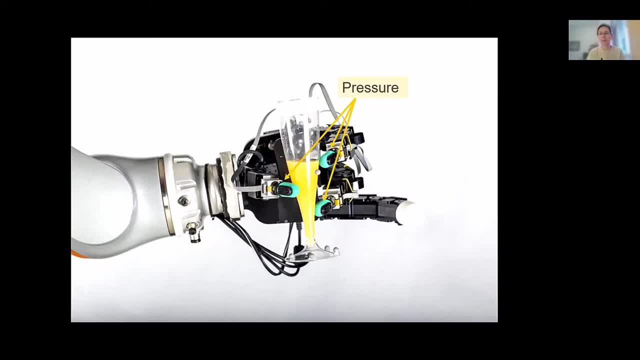 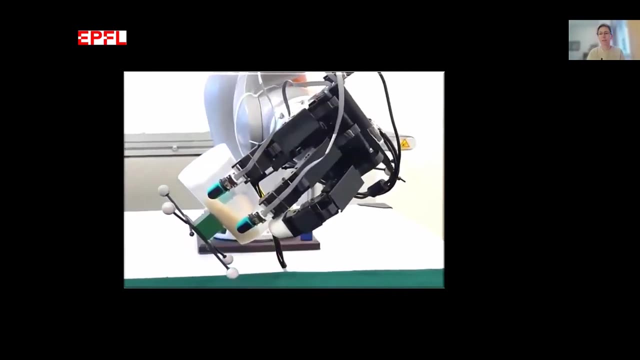 by using pressure information that is measurable. Here we use these sensors, which are called biotechs, that can measure tangential normal force. So let me show you an example of the use of this before I explain how we can do that. So here we are, moving this glass. 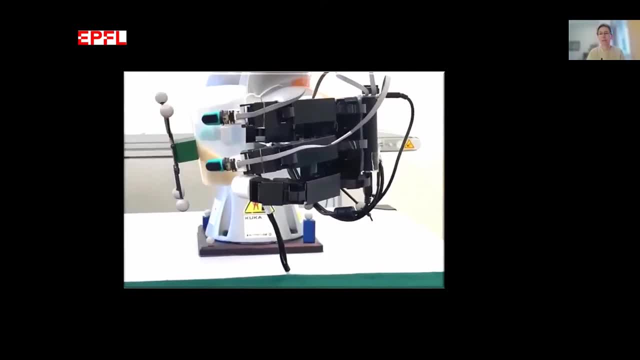 we're just generating a rotation on that glass, but that glass is filled with content, with rice, which is twice the weight of the actual glass. So this generates torques that we need to compensate for. To do that, we need to measure the force. 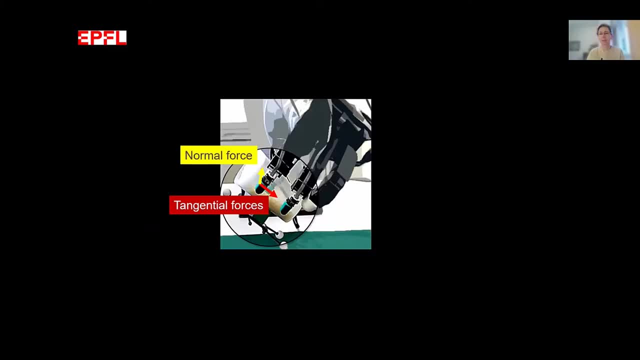 as I said a minute ago. so we need to measure the tangential force and the normal forces and to see how they change as we move the object in space And, of course, we need to use this to generate the appropriate torque. Now we want this problem. 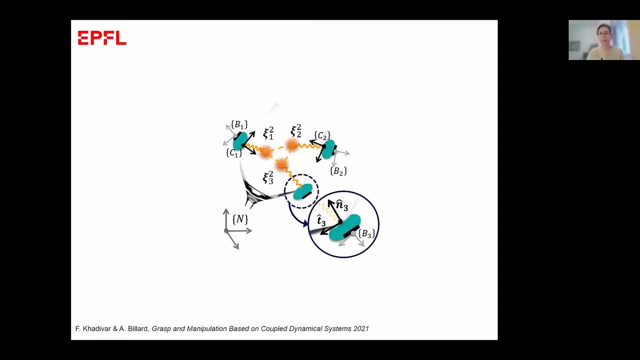 to be as close as possible to the reality. That means that we start off with no a priori on the shape of the object. We assume we don't know the shape of the object. we don't know the weight of the object either. 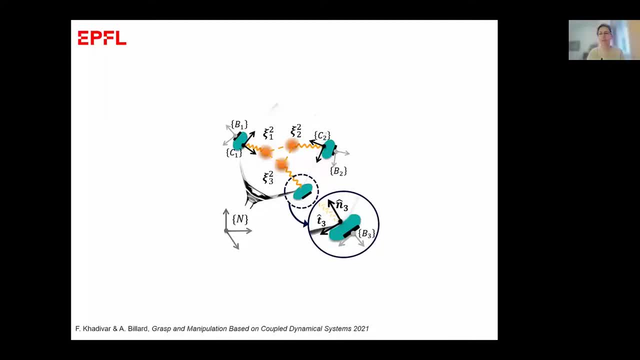 and we need, at one time, to be able to estimate it. Why do we start with this assumption? It's typically because we want our grasp to be generic. don't forget: what I explained before is that we choose, for instance, to choose different grasps. 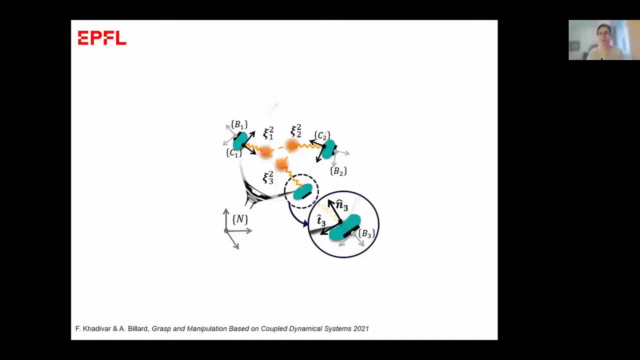 on different objects based on very simple shapes on cylinders or balls, as we've seen before, but we can then generate these as pre-shapes that can close an arbitrary object. So we don't want to know the shape of the object. we want to be able to adapt. 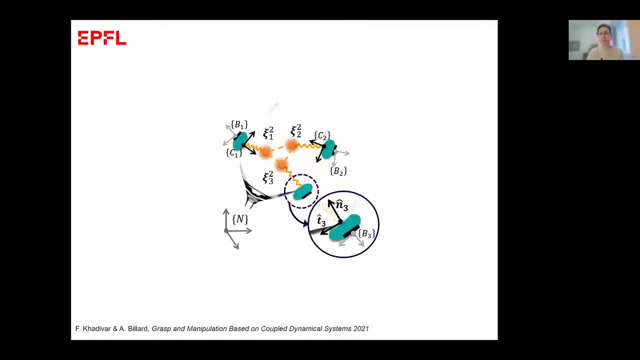 to the shape of the object upon contact. and we don't know the mass because the mass will, by definition, change, as in the previous example I've shown, will change as a function of the change of the content we see in the object. 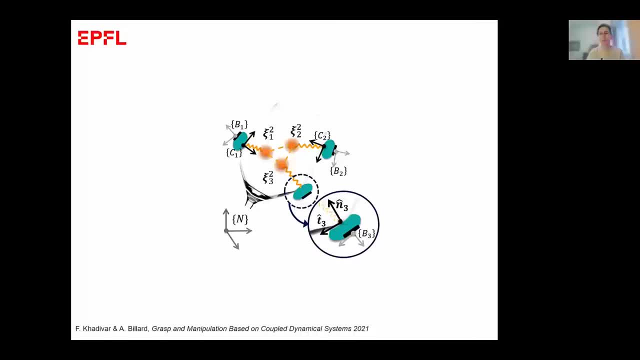 So all we know is the forward kinematic. that means the placement of my finger, and we assume here that the object are already in contact with the. sorry, the fingers are already in contact with the object. So once we have the position of the finger on the 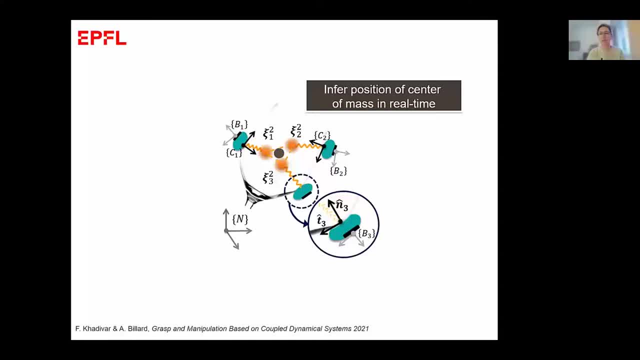 we have the forward kinematic so we know where our finger lie. then we can use this to infer the position of the center of mass In real time. Typically, if we sense only normal force, then we can assume that the and that this normal force. 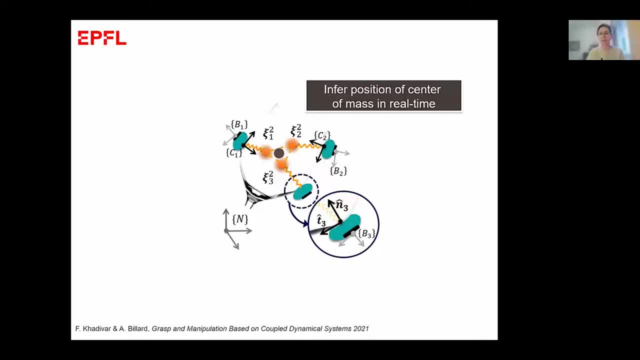 sum to zero or close to zero, that they represent force closure according to the criterion of force closure and they stabilize the object. Then we can infer the position of the center of mass from this, simply this triangulation across the position of my three finger. 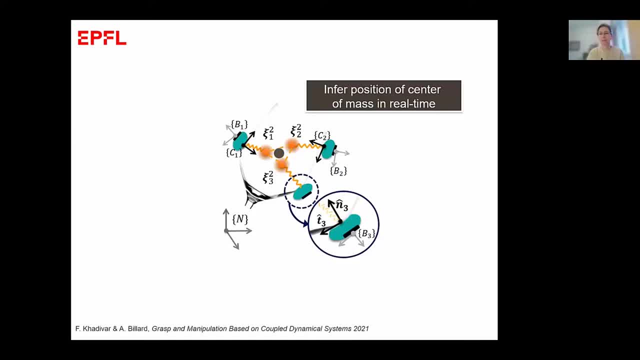 If I sense tangential forces, then I can estimate that this is starting to slip and then have an estimate also of the displacement of this center of mass. Now, when I do that, then I need to immediately adapt the finger orientation to restabilize the object. 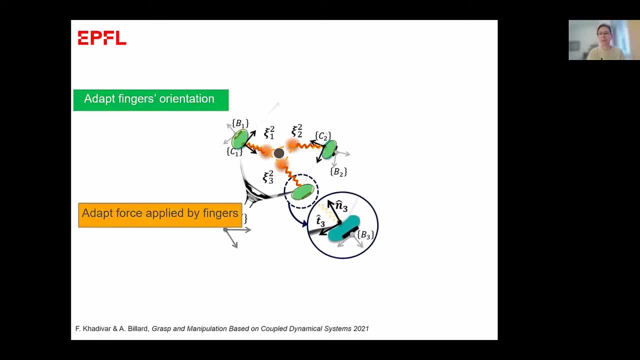 And I also probably need to adapt the force that is applied by the finger to increase the contact force and to increase the amount of normal force, to decrease the slippage that I'm perceiving on the tangential force. So this is what I have at my disposal. 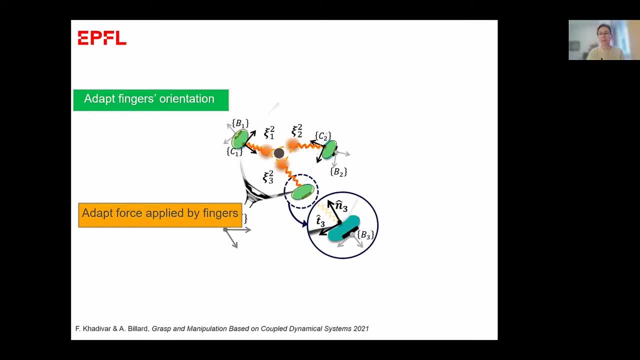 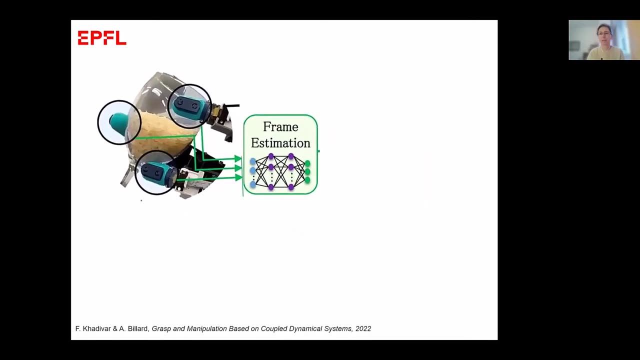 I start with this representation of the object that is given to me by these contact points, these contact forces, and I build my controller based on a sense of how these forces change. So I estimate the frame, the frame from this contact point, the normal. 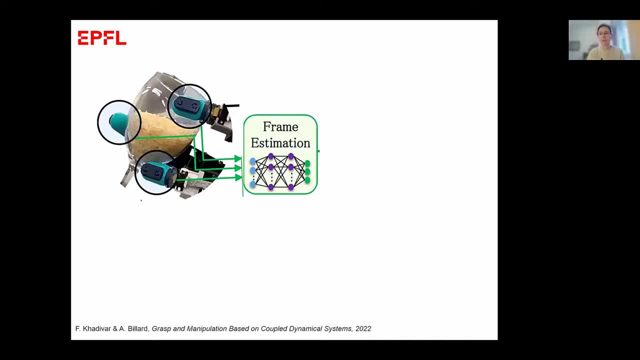 to the surface of my fingertip. I will not explain this in detail, but typically, because the contact points are actually very difficult to represent, there is deformation when we are in contact with an arbitrary object. We also used for this machine learning. 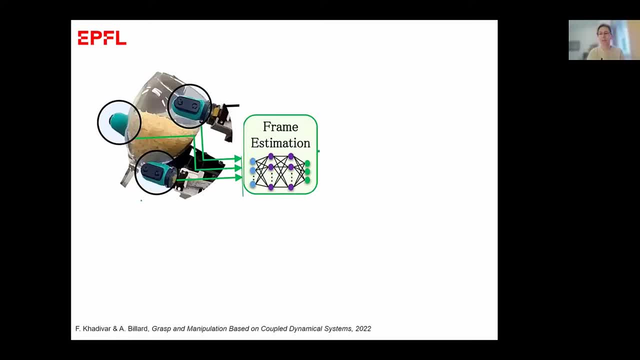 we use a neural network to estimate the relationship between the deformation that we are perceiving at the fingertip, and we have actually 19 electrodes that represent a measurement of the deformation at each of the fingertips, And this can be converted into a representation of the frame. 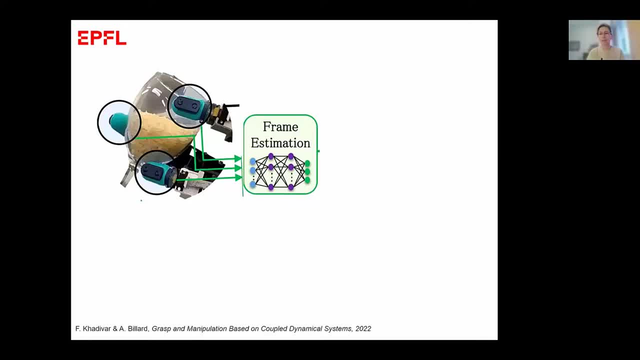 of the normal and the frame of the forces, and the normal and the tangential force. So that's just a quick overview of this. Now, once we have the contact information, then we can use the forward kinematics, as I said, to represent the object force. 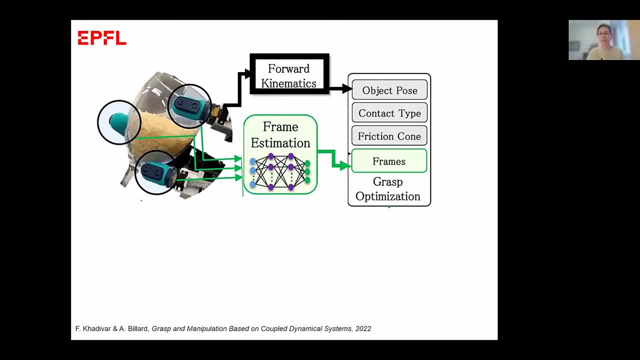 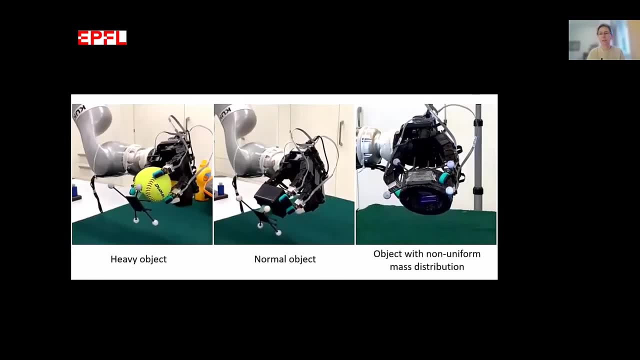 and then compute now the slippage and optimizer. So with this representation we can at one time adapt, And of course it's difficult to observe, because here you basically don't see the adaptation of the force, but you can see the adaptation. 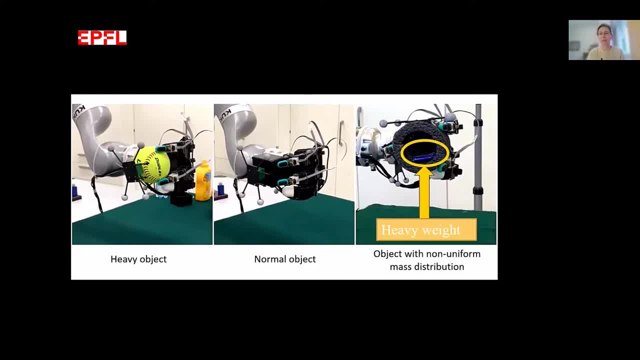 of the finger position And these three objects are difficult to manipulate: The left one because it's fairly heavy for the hand- it's close to the maximum weight that the hand can hold- And the one on the right hand side is tough because we've added: 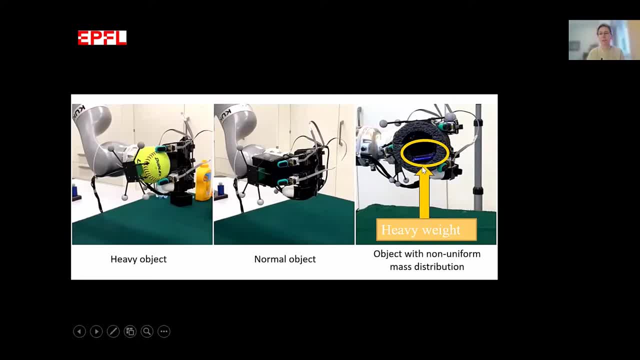 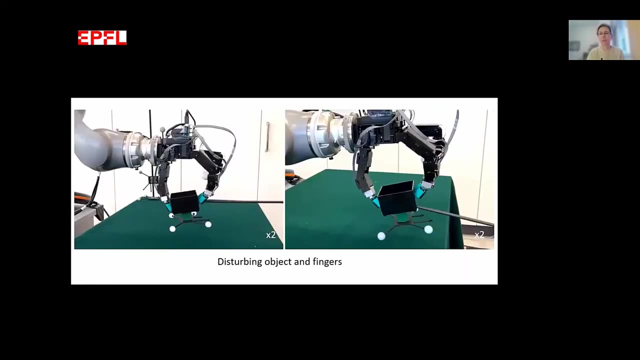 as you can see here, a heavy weight. It's actually a little battery which makes the object twice more heavy on that side than the rest. So it's a non-uniform mass distribution and we can adapt the grasp. Interesting also is to show 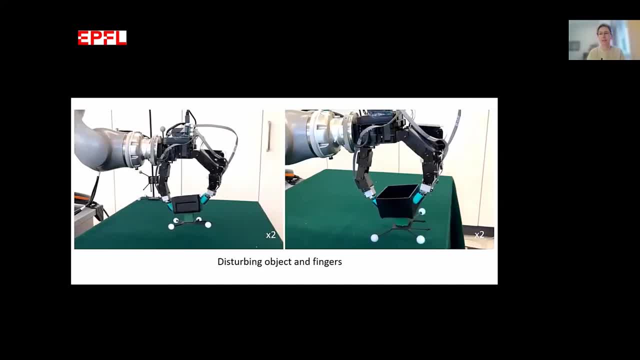 that we can adapt the grasp at runtime. This is where you can observe the adaptation of the rotation of the fingertip on top of the adaptation of the force when the object is subjected to arbitrary disturbance, as we see here. I'll just play the video once more. 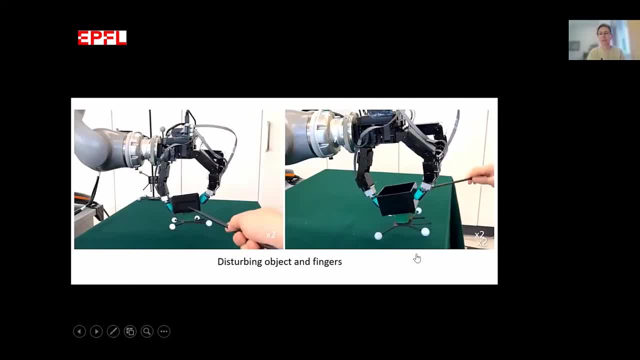 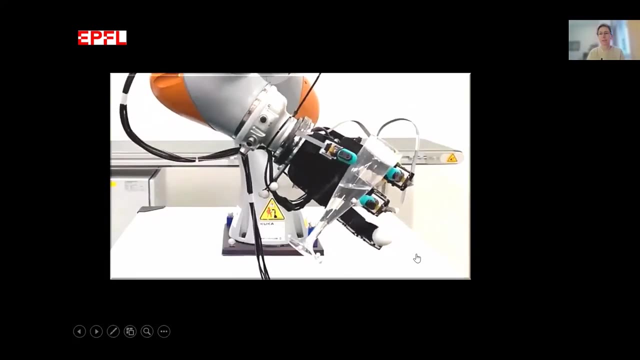 So we can generate small perturbation pushing the object that generates both translational and rotational displacement, and have the hands compensate and rebalance the position and the weight. Finally, this is, of course, my major goal in this work and that's what we set. 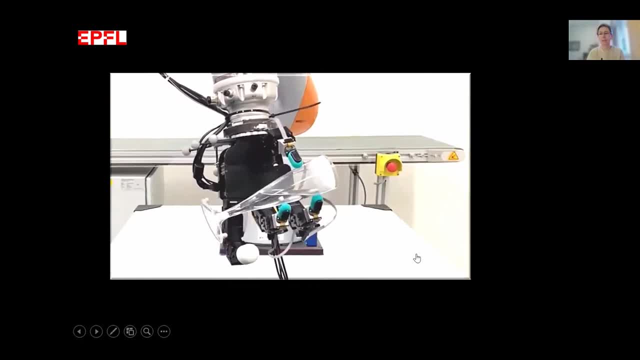 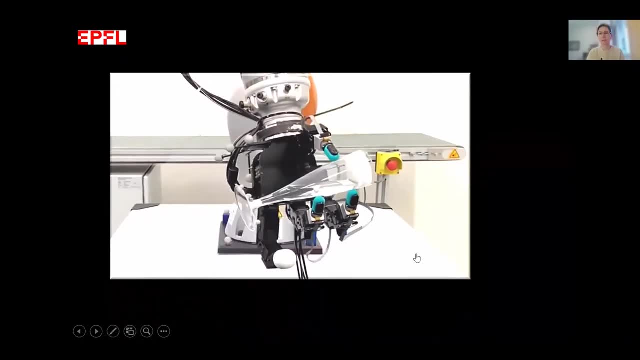 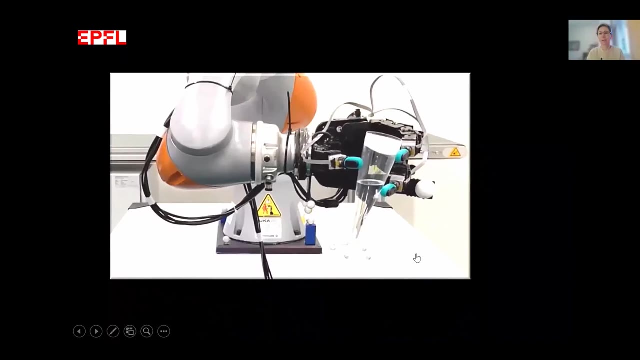 really all our efforts towards was to be able to balance this particular complex object. It's complex because the shape itself is complex. It's complex also because the object is very slippery and because, finally, the weight in the object is three times the weight of the actual object. 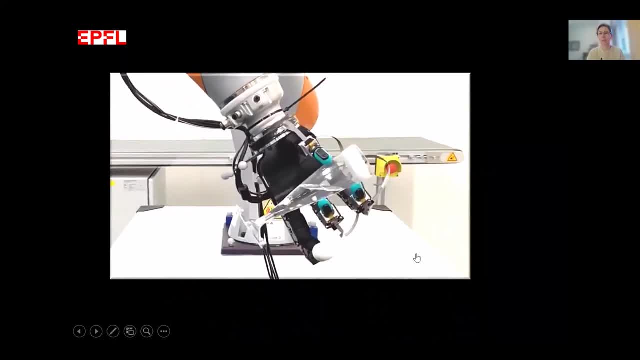 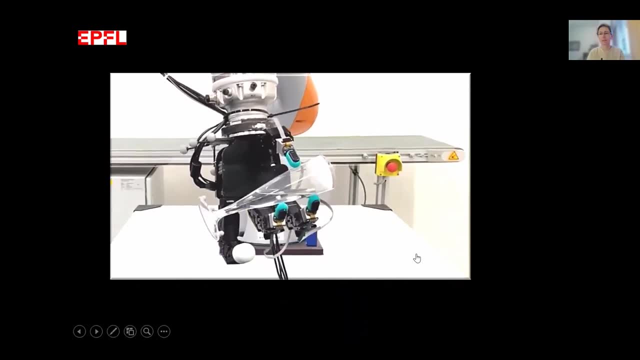 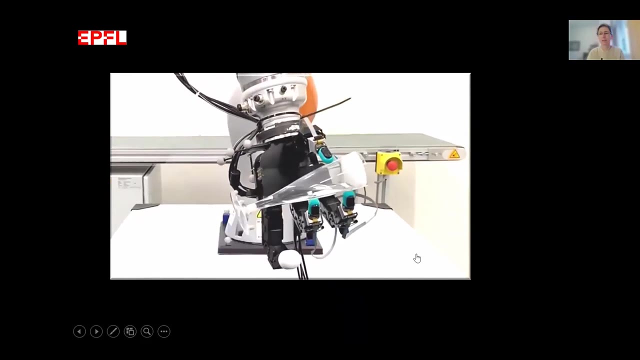 So when you rotate the object, the fluid here generates a lot of changes in the mass distribution over the object, which generates, as you can see, some sort of slippage or rotation of the object inside the finger and you have to make sure. 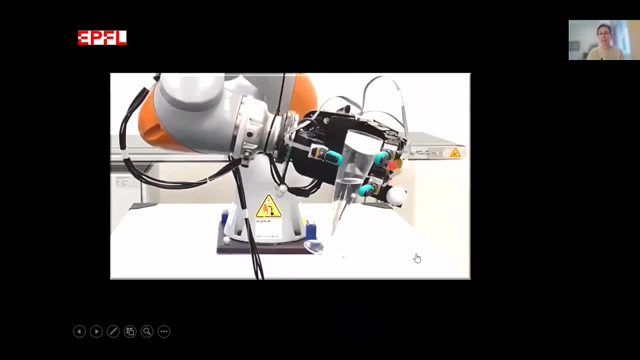 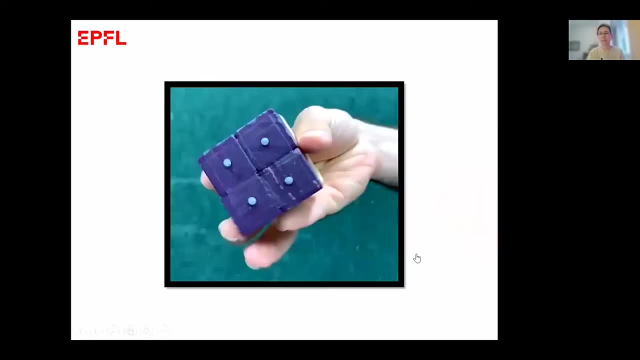 that, even though you allow for some of this, you're still keeping the object within the foreclosure cone of your finger. Now, lastly, for this last part of the talk- and I hope I still have time for this- I'd like to talk about. 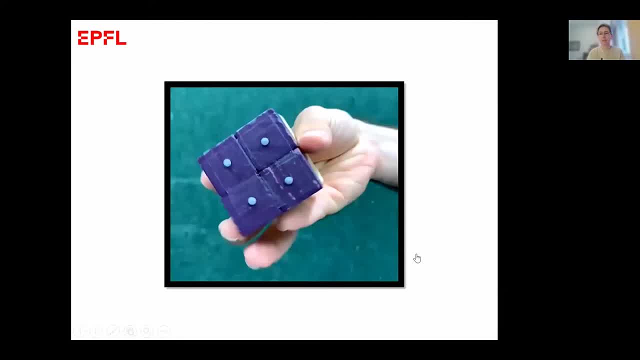 one more step towards this human dexterity, which is then to not only adapt to displacement of the weight of the object as you are moving it, but also to be able to do what is called in-hand manipulation and to rotate your object inside the hand. 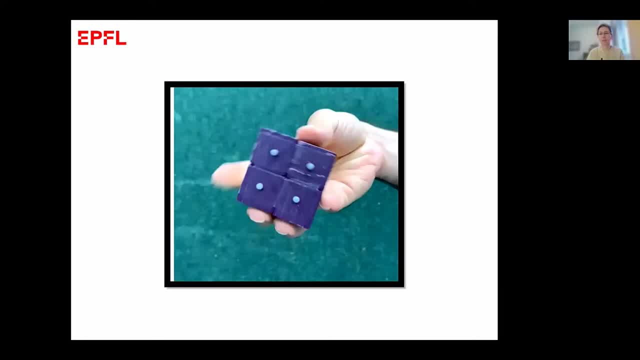 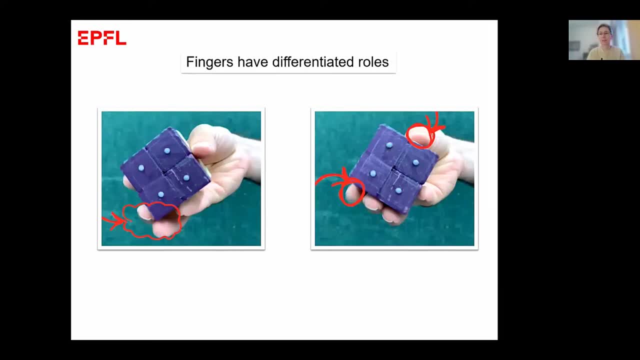 So we took once more inspiration in the way that humans do that and we look more carefully at the way that humans manipulate such objects. So if you pay close attention, you'll see that there is a distribution of role across fingers when you do that. 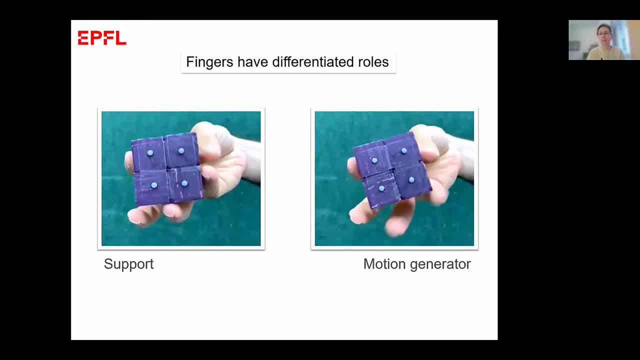 Some are used as support for the weight of the object, whereas others are used as motion generator. So we have again. I'll just play here. we have the support finger, which are the bottom one, and then we have the top one. 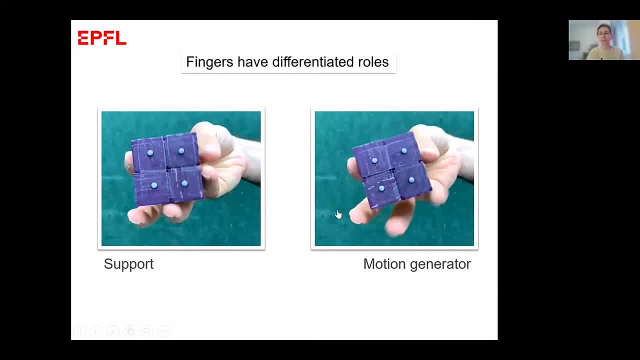 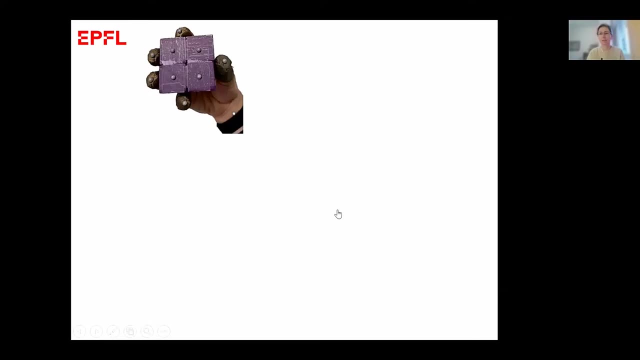 which are being used to generate the rotation on the object. Now I could handwrite this role distribution or I could discover it. We took the avenue of trying to discover that automatically. So we start with human demonstration. We track the motion of the finger. 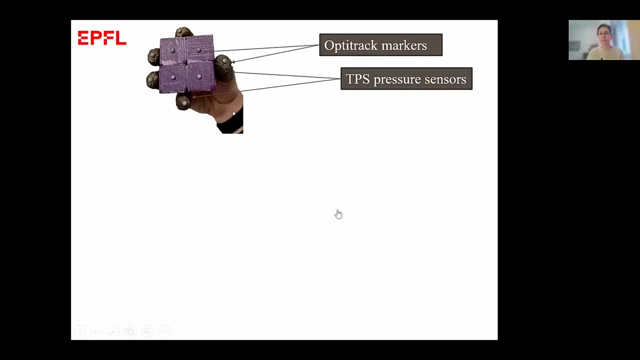 We track the change in pressure information as the finger move, generating this motion around the object. And, of course, the combination of the motion of the hand, the motion of the finger and the pressure sensor allows us to determine which of the finger play a role as a support. 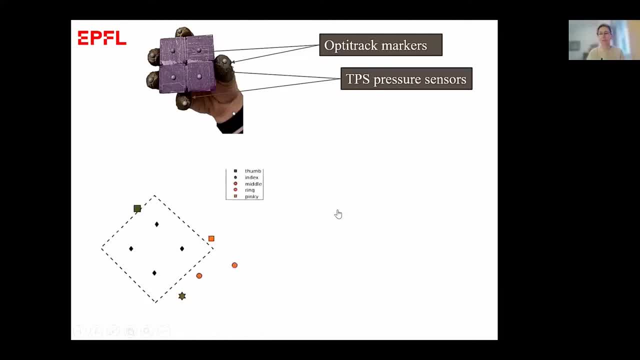 carry all the weights and which one generate motion. So this is now a simulation of the tracking of those fingers. So the marker of each of the finger are represented here by those different points and you have little square, little round, little star. 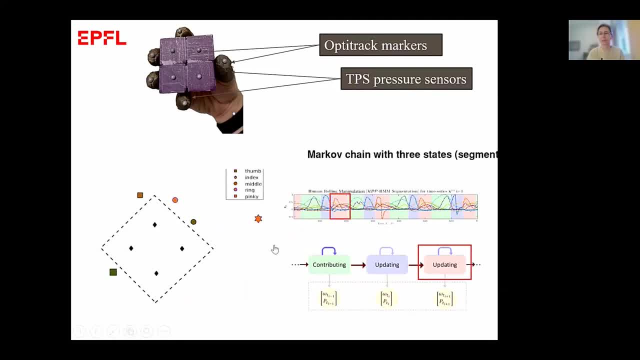 And each of those then can be extracted as a sequence of motion, which I show on the right-hand side. For that we used a representation as a Markov chain, So we could use what is called hidden Markov model. that allows you to estimate first. 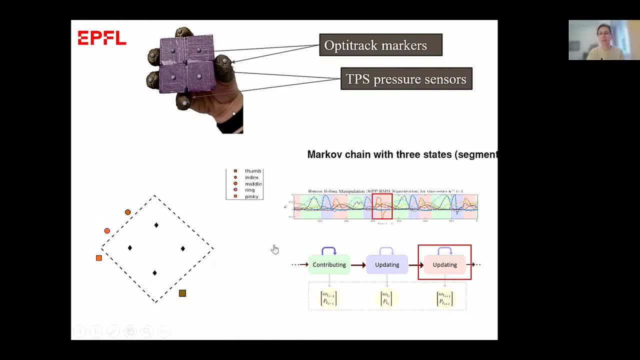 the number of underlying states in a particular motion. Here in this in-hand manipulation, we can identify three states which can be labeled as there are states during which the finger contributes to support the weight And there are stages between, during which they update, and they update in two sequences. 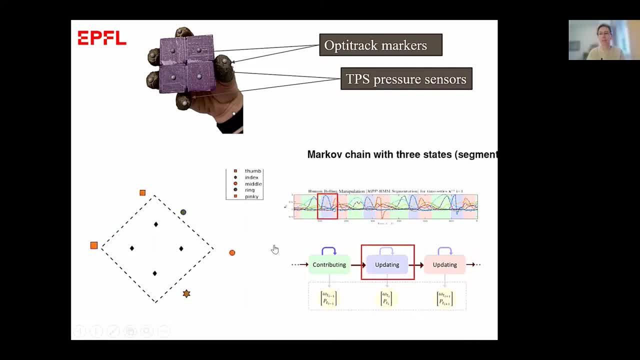 They update the thumb, and then they update the index, typically, and the middle finger, one after the other, to generate the motion. So I'm going to go through those stages in more detail for you to appreciate how we can then turn that into a control system. 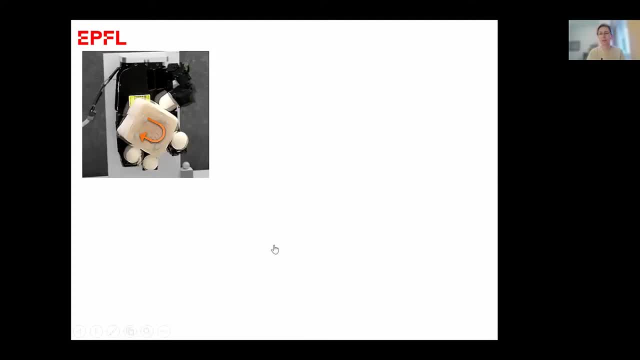 So if we look at just a close motion here is already looking at it from the standpoint of the robotic hand that we will use for control. So we start in a certain configuration and then we need to generate a motion. So, to generate a motion, 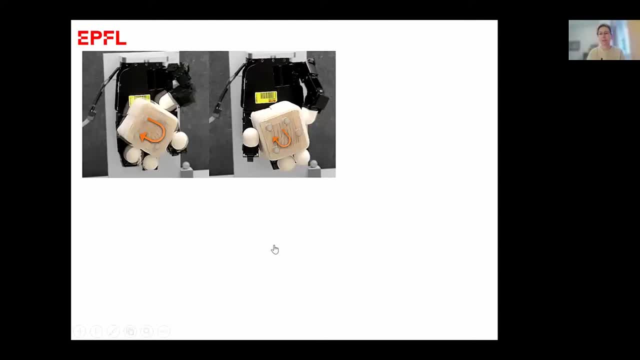 which is here just a simple rotation, an anti-clockwise rotation. what we need to do is to move the thumb and the fourth finger in opposite manner, So you see that there is a motion from the thumb to this particular location, And then we can. 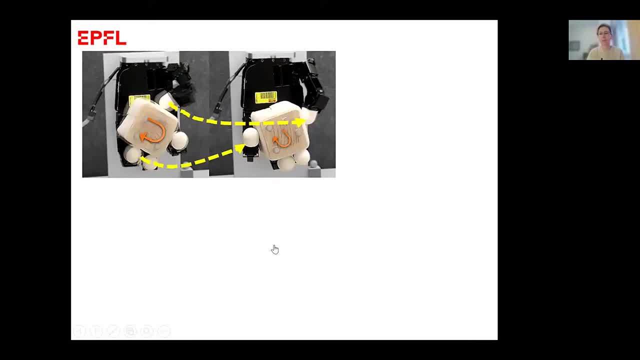 move the thumb. and now for this last finger, the fourth finger, the ring finger of the allegro hand. that needs now to rotate in the opposite manner, And we also need to generate a little bit of a motion of what is a support finger. 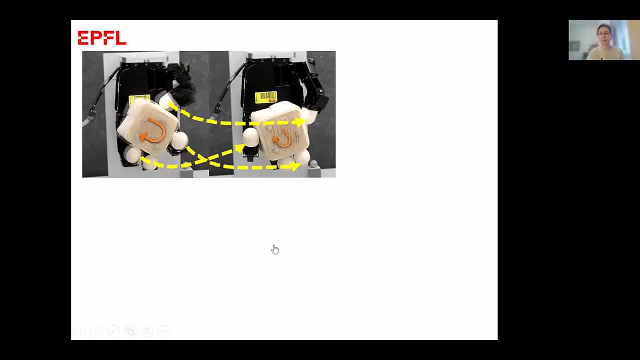 So this finger is probably the most challenging one because it has to both move but also support most of the weight. Now we can schematically represent this as our fourth finger here to act as support. They have to control and rebalance the weight, Whereas the other three are. 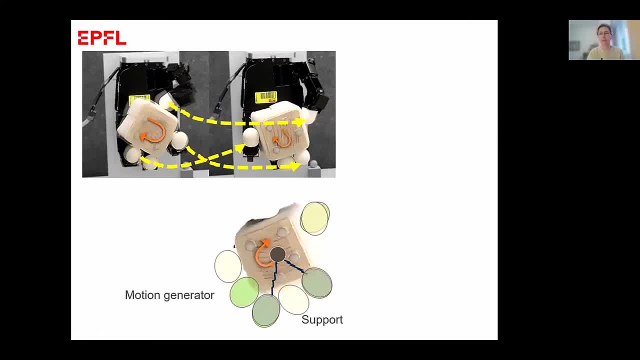 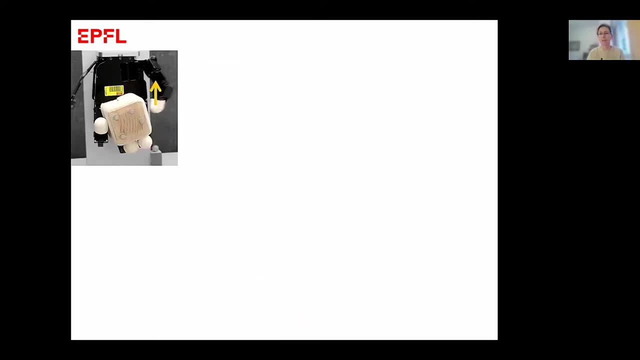 so, whereas we have three fingers that are motion generator- and here I'm just representing again what we need to do to control for this simple motion- Here we're only doing a small part of the motion. The most challenging part is the one that I illustrate here. 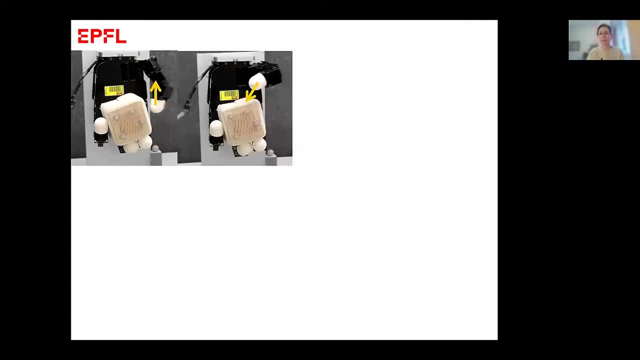 is when one of the finger has to leave the object to come to another position, And then the other finger has to move and then apply force to generate motion. While it does so, the other finger stay put and then, once it reaches the object, 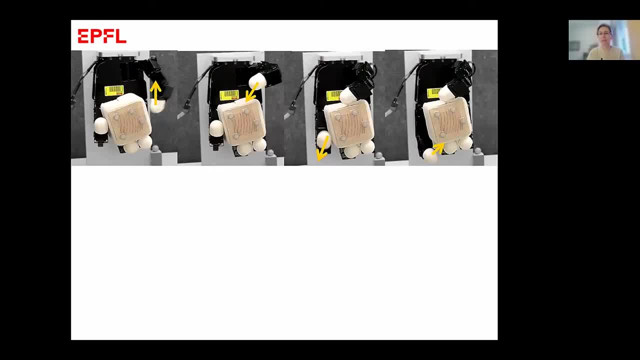 then, for instance here, the fourth finger has to move and then join the other, But as it does so, the top finger or the thumb will actually apply pressure to generate a motion, and they will do that in coordination. Here I will focus simply on explaining the motion generation. 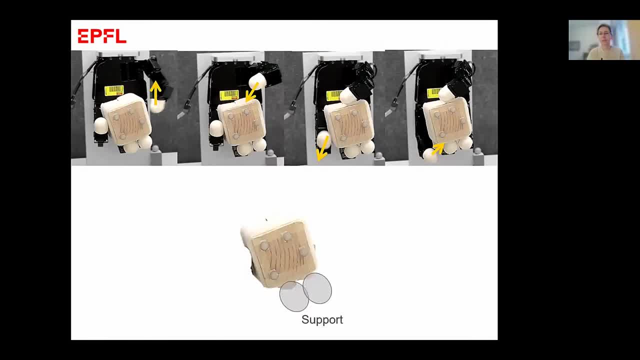 So let's go back to our schematic. We have two support fingers and we have now the two motion generator fingers To generate this lifting motion. what we use is something we've used extensively in my group, which are called dynamical system generators. 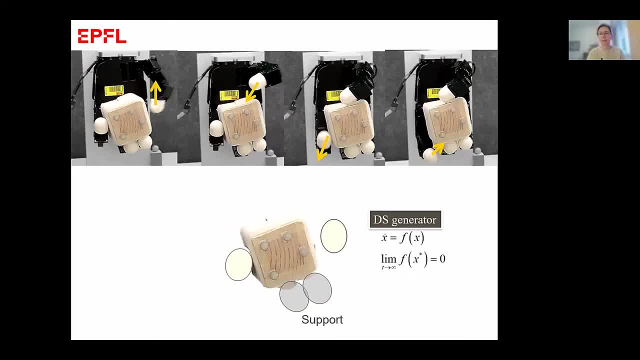 These are differential equations which have particular properties- They are stable at an attractive point- which are represented here, which is the point where we want the finger to reach. Now, the nice thing about this DS generator is that it's very flexible, So we'll see that in the next video. 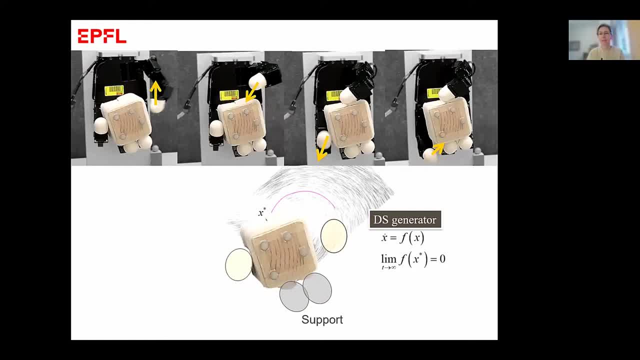 is that it will always recover from perturbation and be able to come back to its attractor, even if it's pushed away from its goal. So once we have this, then there are an infinite number of trajectories we can follow, and here is one of them. 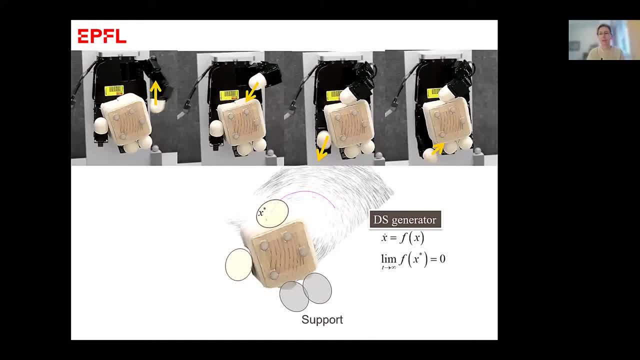 depending on where we are, that will lead us to this attribute. So we have such a DS generator for each of our fingers that allows us to generate the motion to the desired next point. Now we can sequence them through this HMM and have this sequencing of motion. 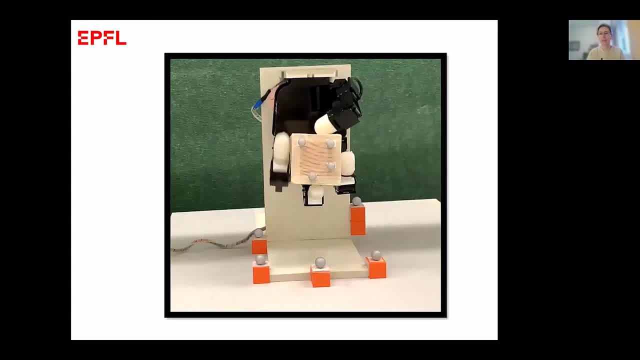 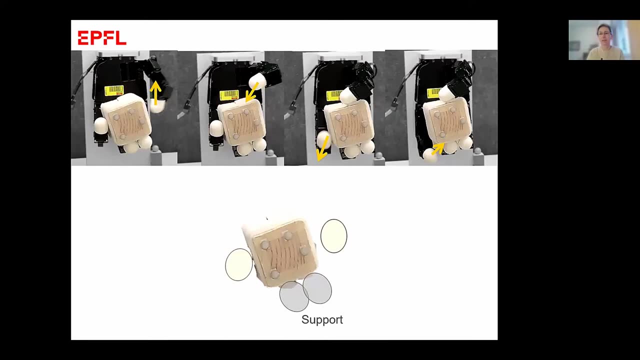 So this leads to this nice demonstration, So we see that we can rotate the objects inside the finger, have this nice sequencing and coordination. I mentioned coordination, but I haven't explained how we coordinate. So let me first explain to you why coordination is crucial. 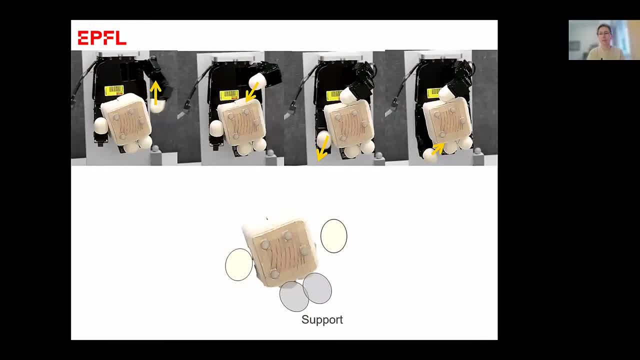 Imagine that I start with this motion generator that I've presented before. I move a finger and boom, it's intersecting, and the second finger goes and moves with a sequential temporal sequence, without waiting for the first finger, the thumb here, to reach the object. 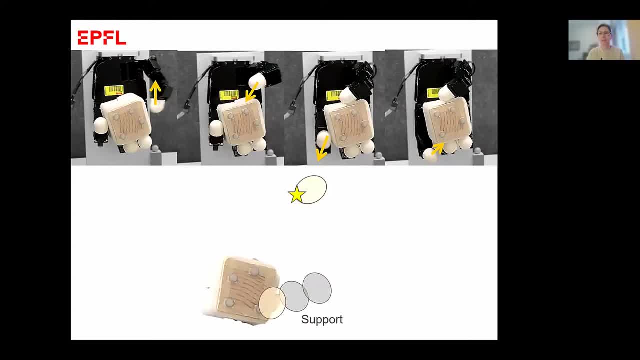 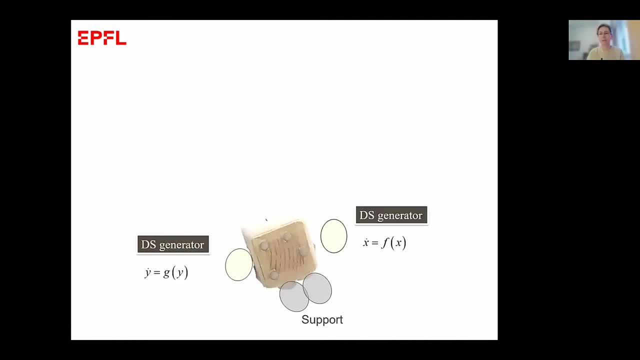 What happens is that obviously the object falls. So we need to have a coordination and we need to make sure that this coordination is embedded in the controller. I'll go very quick. We can do that in close form. This is extensive work, also of my line. 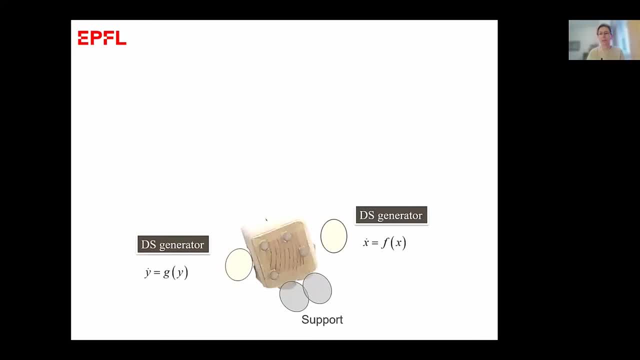 that I will not go through detail. but as opposed to use two separate DCS generators, one for the finger denoted here by x and one for the finger denoted by y, we can make sure that they are coupled and in dynamical system control. 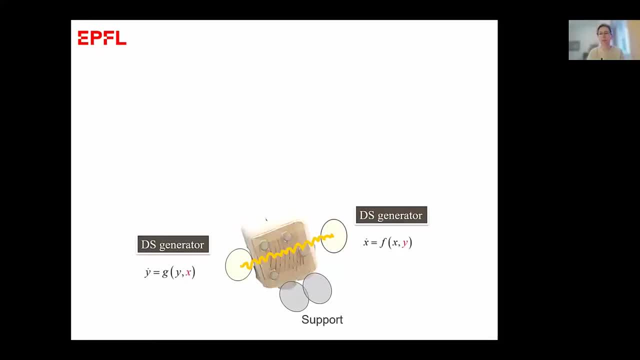 that means that each of the variables becomes a codependency to the other dynamical system. We can prove that these two systems, once coupled, will both reach the retractor asymptotically in sequences. I will not go through the social proof here. 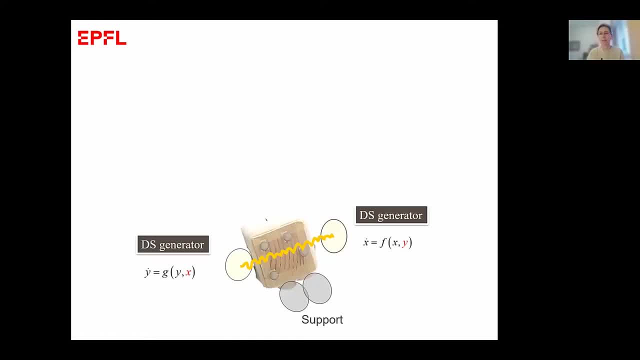 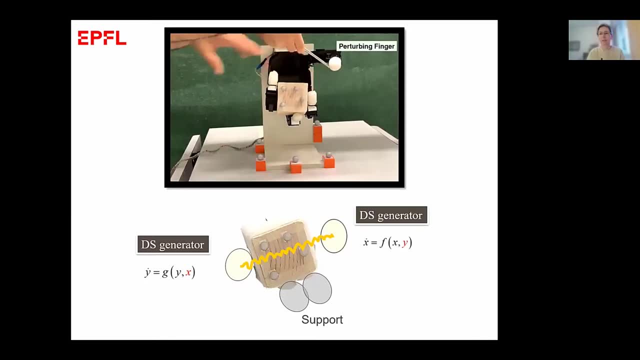 Once we have this, then we can generate all sorts of very nice robustness against perturbation. I'll show you here a couple of examples. You can stop one finger. You can move the object. As you move the object, you simply move the attractor. 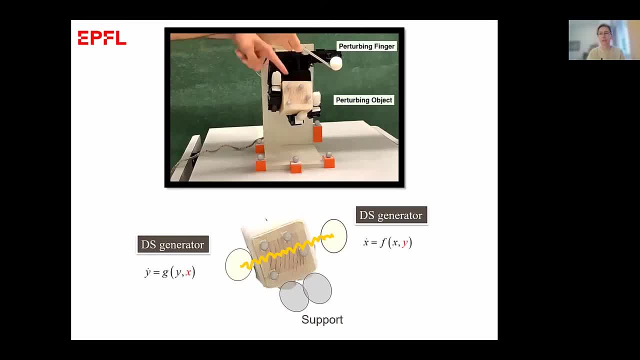 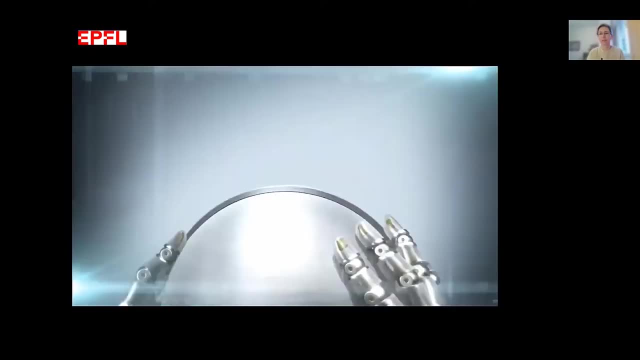 but the system remains. coupled to this different attractor, You have this nice preservation and robustness to both the displacement of the object and the displacement of the finger in coordination With this. this will be the end of my talk. I'll just give you. 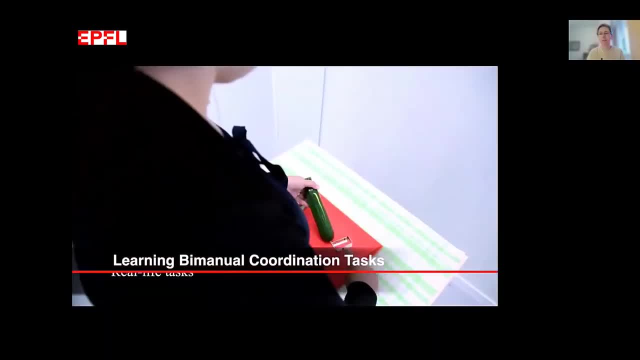 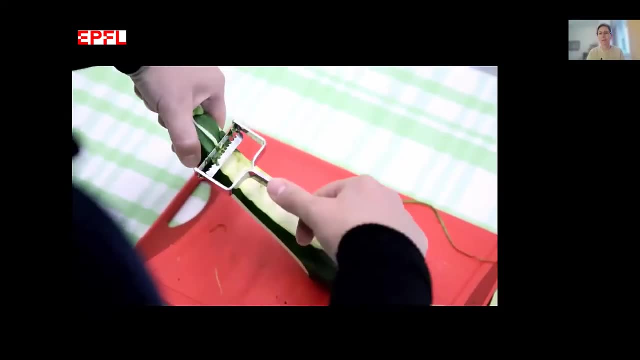 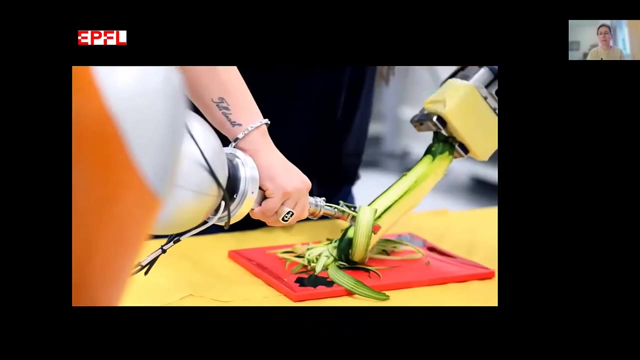 a very, very brief overview of other work that we do in the lab, which we will not have time to discuss in detail. We have done extensive work on manipulating deformable objects, typically fruits and vegetables, learning from demonstration, using here also computer vision. 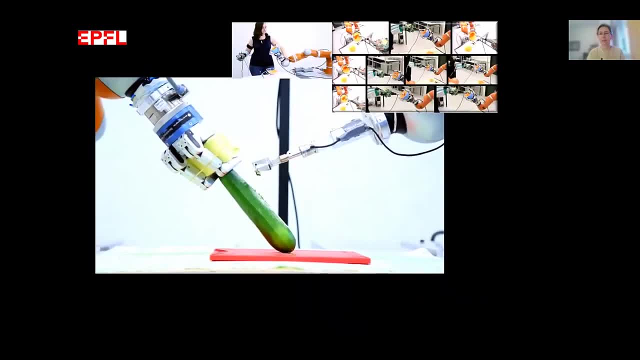 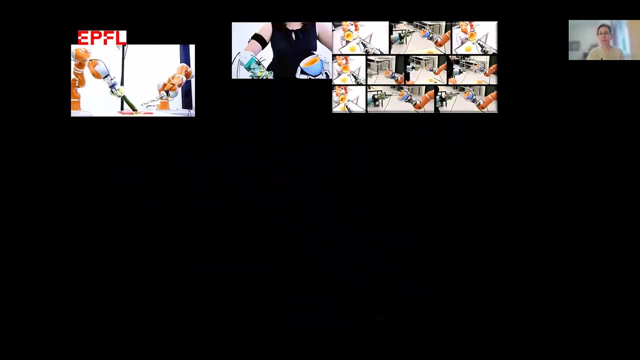 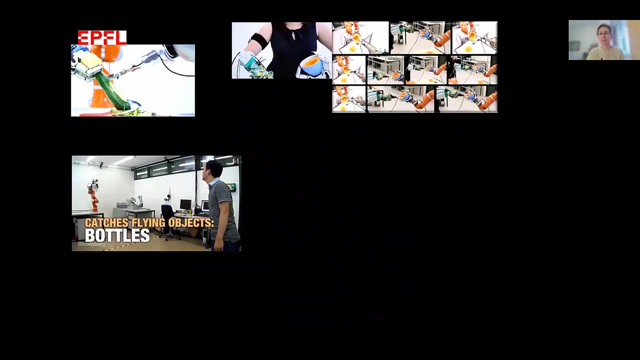 to be able to extract changes that are generated on the object to generate different motion. We've done it also for different fruits, as we see here, than typically for scooping melons. Now, the interesting part when you do that for these vegetables: 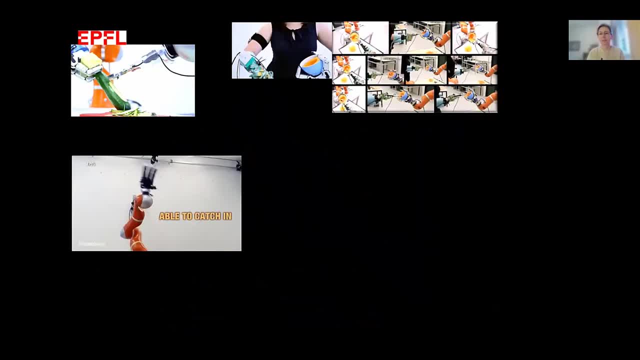 is that no two vegetables are the same. Now we see other examples. A lot of work that we've done was on extremely fast computation for catching objects in flight. We've done many different examples of this, which were then ported for bimanual coordination with humans. 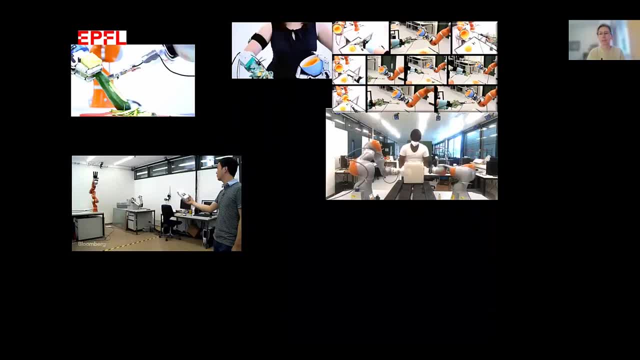 as we see in this example, having flexibility and adaptability of bimanual motion of the two arms and also bimanual coordination of forces, which we then used also for generating typically handover motion from a robot to a human, Adapting to the motion of the human. 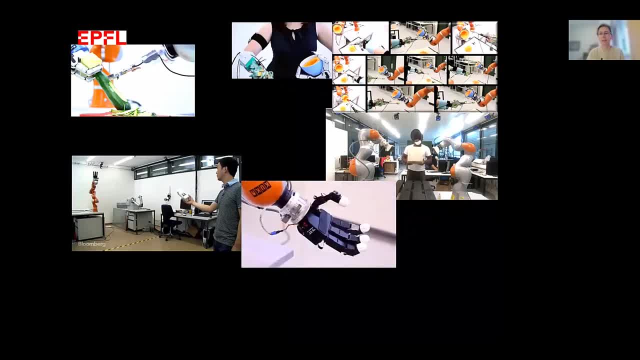 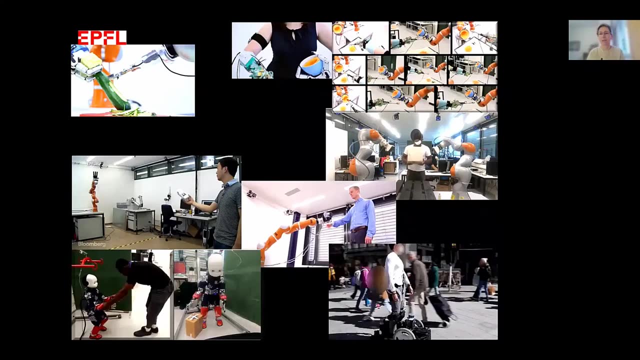 adapting also to the pressure applied on the hands. This is a coordination between hand closure, finger closure and motion of the arm to enable the robot to adapt to both the motion of the human and the motion of the arm. And of course, we've also looked at 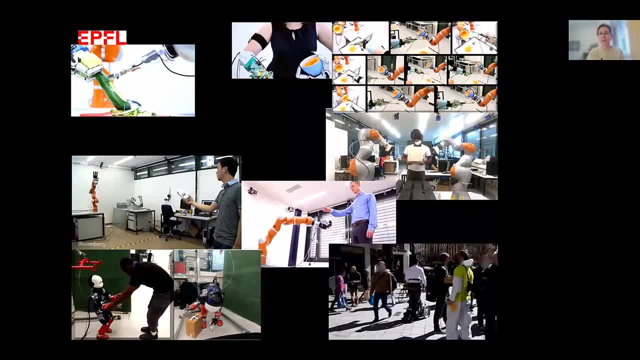 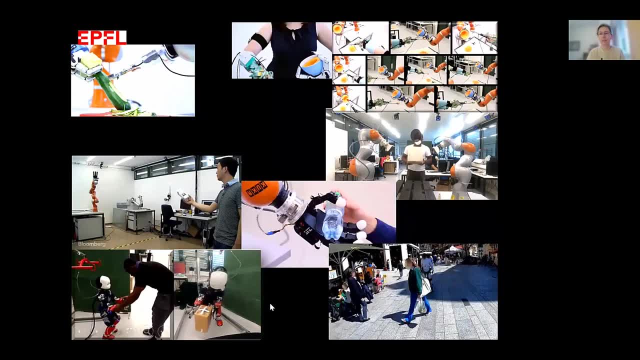 many other interesting problems in robotics, which are navigation, be it navigation of a wheel-based platform, as we see on the right-hand side, for navigating in crowds, or navigating a human robot in coordination with a human. And perhaps the one that I loved most: 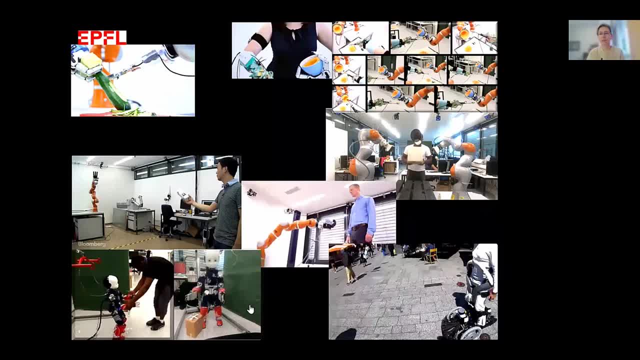 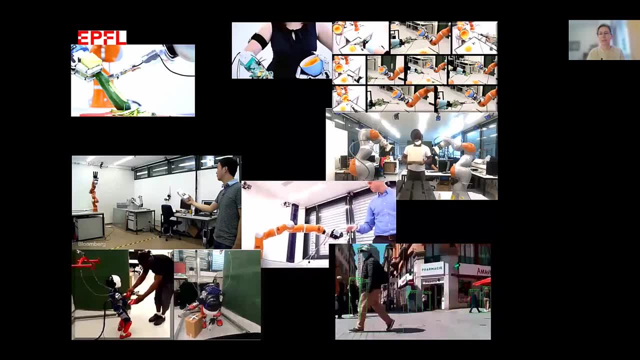 which I'm highlighting here in the middle is this one where it's a bit similar to what I presented for the hands. It's here using the entire number of degrees of freedom of a human robot to go down and pick up objects and lift them. 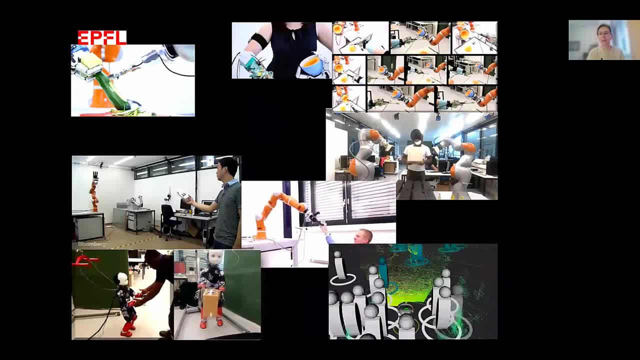 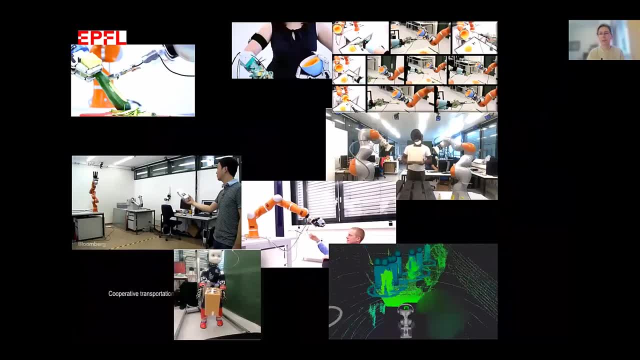 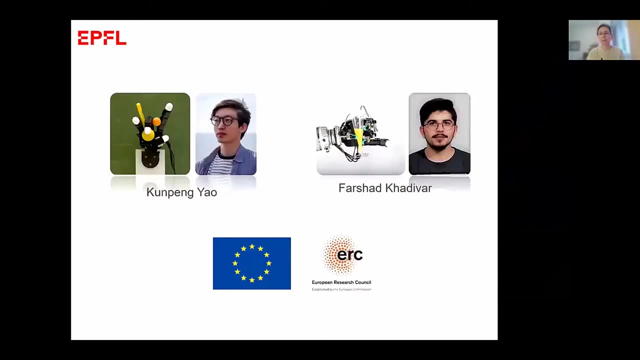 So balancing the force to stabilize the object, as well as exploiting the entire dexterity of the full body control. With this I want to close the talk. I want to thank first Kenpeng Yao, who has done all the work, the beautiful work. 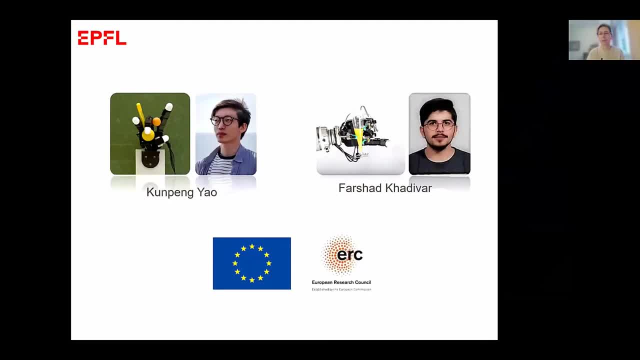 that I presented here on picking up multiple objects inside a hand, and Farshad Khadivar, who did the wonderful work on balancing the weight of an object in hand and the in-hand manipulation that we do. Thank you very much for all the work. 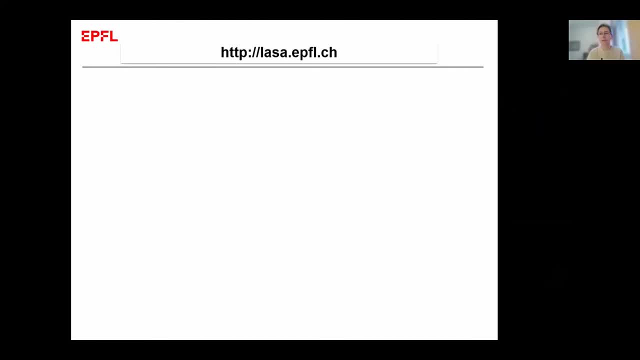 that I presented. The work that you've seen, is all documented on our website. We have a source code for most of the control system that we developed. We have tutorials. We also have all the publication and videos that are freely available, And I also want to thank 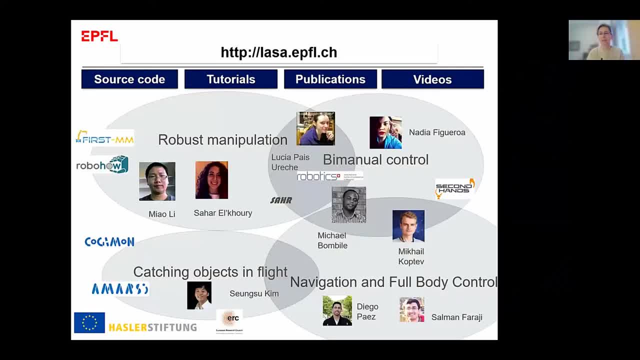 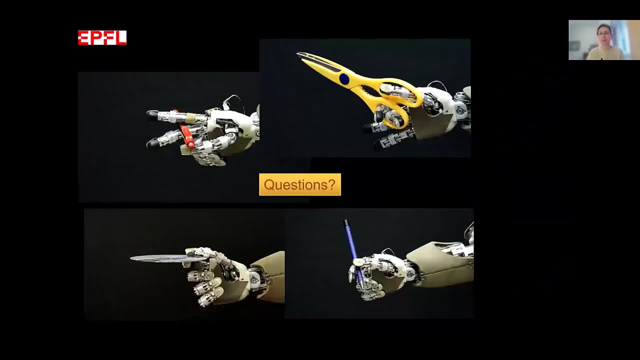 Thank you. Thank you, And I'll close here. I'll ask the chair if the chair wants me to stop the full screen. OK, yeah, Thank you very much. Thank you very much. Let's give her a round of applause. 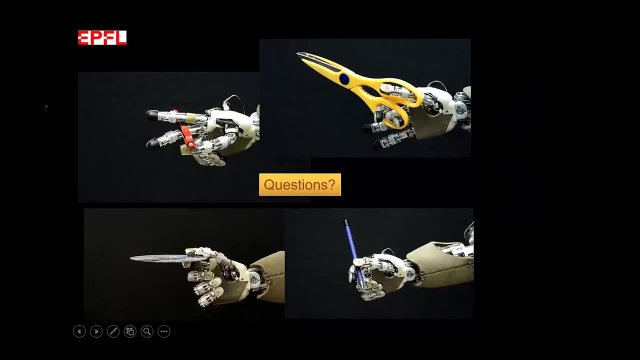 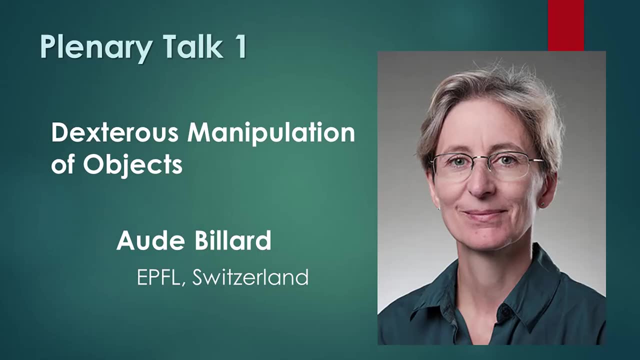 Yeah for excellent presentations. Yeah, it's a little tricky. We have quite a few people on site and we also have a lot of people online. I like to give equal opportunities to both groups of audience, So maybe we can begin with the people on site. 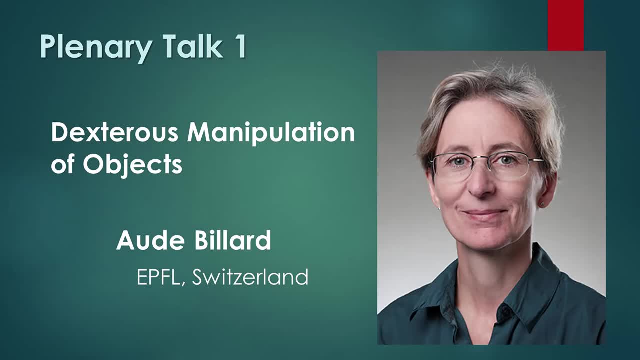 To just ask a question or two. Yeah, Any questions from the audience here. Yeah, that's fine. Hey, Professor, It's a great work. My question is: if you want to grasp a very strong shift? it's very strong. 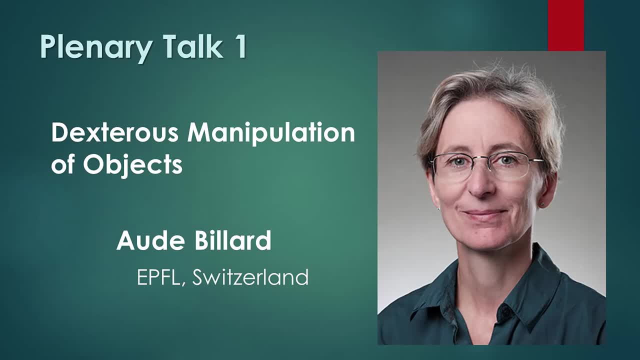 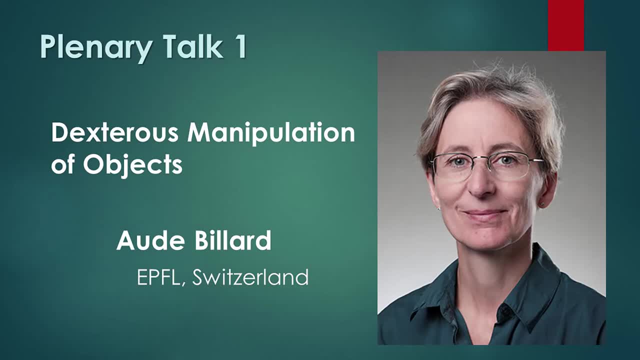 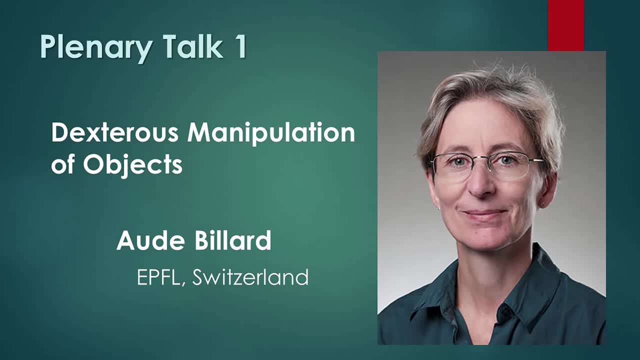 or special sequence I mean to get at. this pattern or sequence is based on the computer real-time computation or is it better to use a human use like a demonstration to show how to grasp it? Which one currently is your life? Yeah, 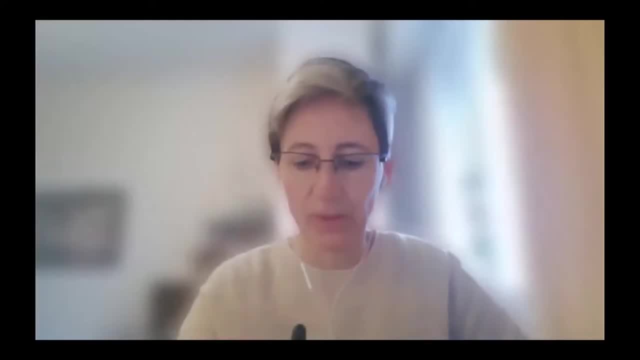 Thank you for the question. So it's difficult to say. I think using the human as a source of inspiration is important in my view, but it stops there. It's really essentially a source of inspiration What we- I mean the road that we followed. 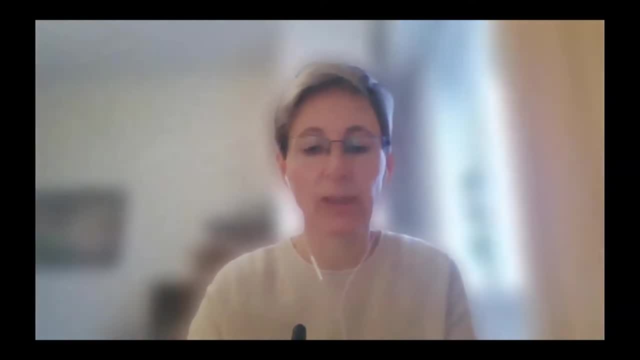 was then to turn that into an actual optimization where we can learn ourselves for the kinematic of the robotic hand, Because, you know, usually the robot hand is not exactly the same as the human hand, So it's not as if you can easily port. 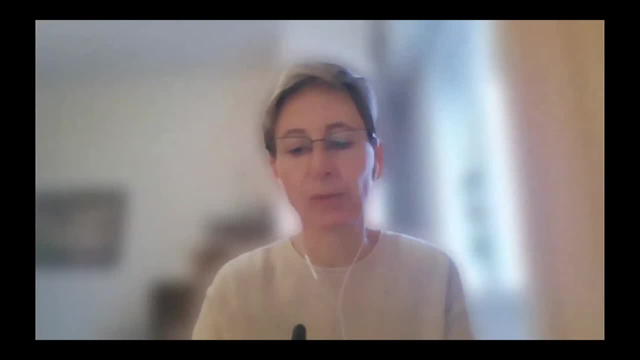 what you've seen in the human to the robot itself. You can take inspiration in the sense that, okay, here are the typical complex grasps that the human can do, But now what are? you know what are the range of feasible grasps? 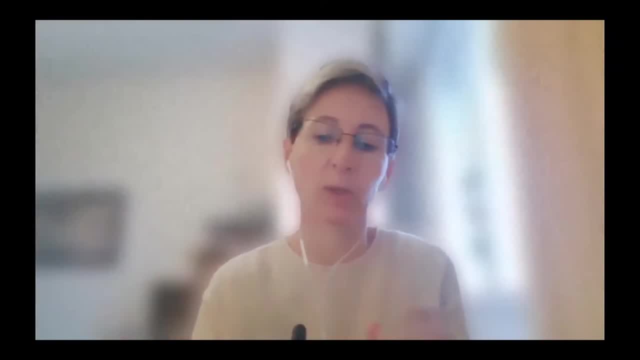 that this particular hand, with this particular kinematic, also with this particular dynamics- because the robotic hand will have different dynamics, will have different strengths across the fingers, different from the human- There are things that you have in the robotic hands which are better than the human hand. 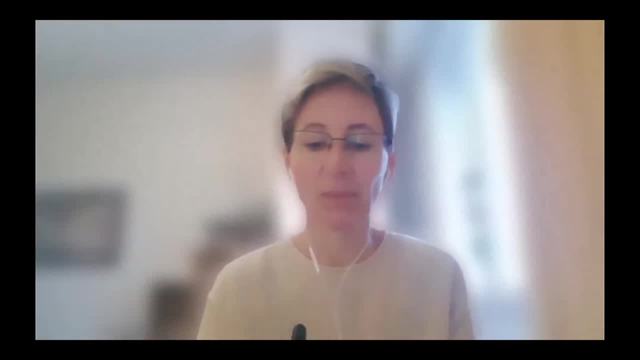 and other things that are less good. I'll give you an example. Usually in the robotic hands, the length of the finger. maybe I'll share screen once more. Why don't I do that? So I'm not in full screen mode. 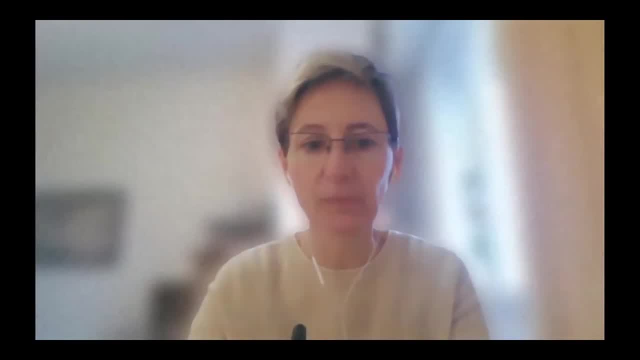 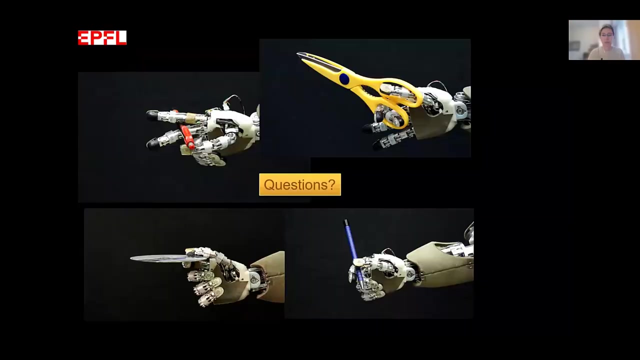 So let me just go back and share to you. I like that. But what I mean to say is that the fingers in the human hands have different lengths, So typically what we call the pinky is smaller and the okay. there is a screen overlaid. 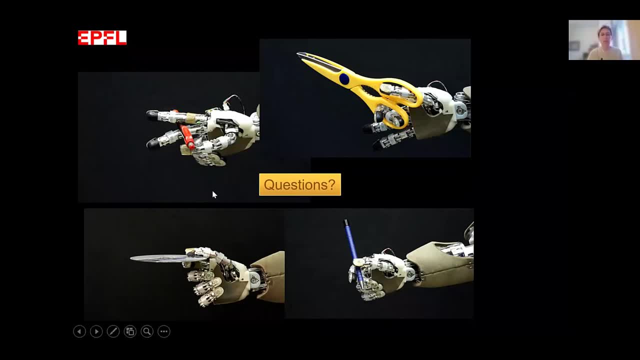 I don't know if it's the same for you. The pinky finger will be much smaller, The thumb will be smaller And then the. you know, the middle and the other two finger index are about the same size. Most robotic hands have actually identical lengths. 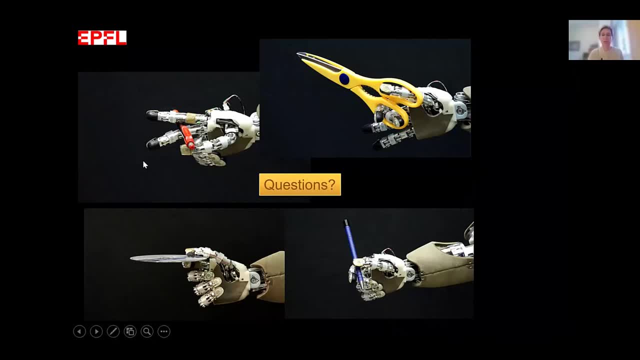 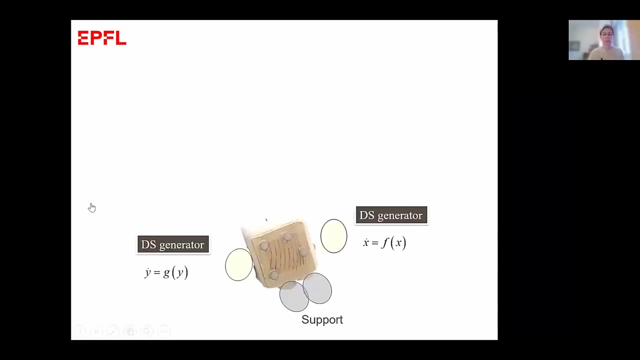 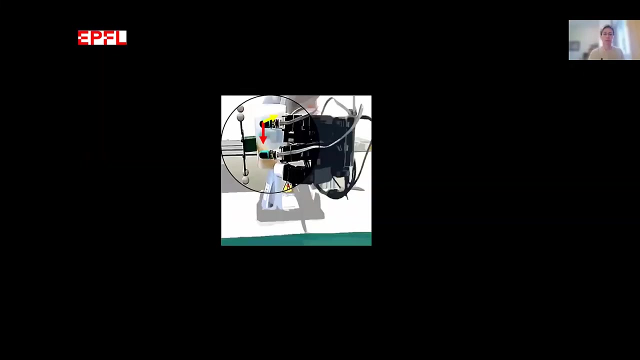 So the mapping is not that easy, And that's a weakness, but it's also a strength, because that's why it's easy for us. If I go back to the very first example that I showed, when we grabbed all the different objects, we can pick up objects here. 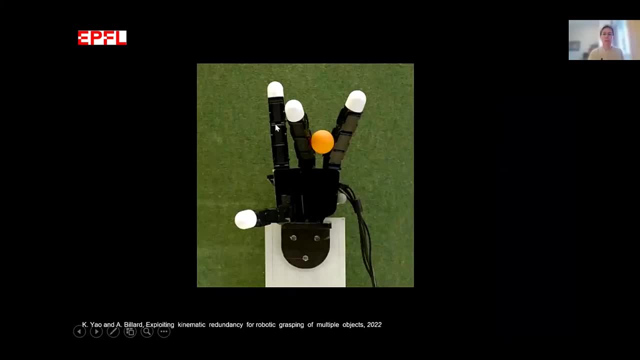 You see, between these two fingers, as well as, let's say, the index and the middle finger, or the ring finger and the middle finger, in that robotic hands, actually identical. There is no difference between those because they have the same lengths, They have the same number of degrees of freedom. 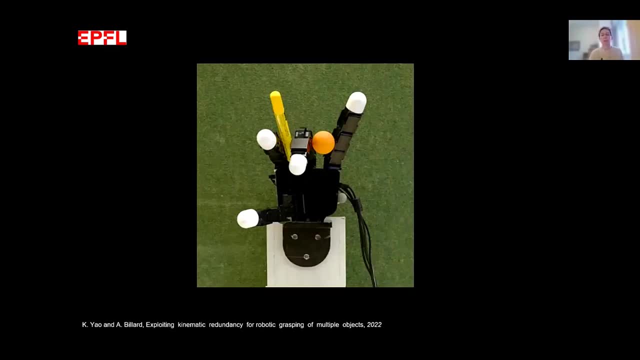 They're also moving the same way. So this is a long answer to a short question. So I'll just summarize: Human inspiration, yes. Mimicry, no. I think we have to still exploit the strengths and the weaknesses of each of the hands. 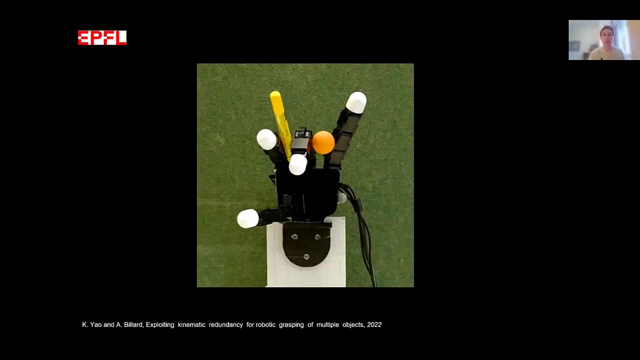 in such a way that we can do with the robotic hands as dexterous motion as humans, but possibly in a different way. Okay, good, So maybe I'll give an opportunity to somebody online. You can either type your question in the chat box. 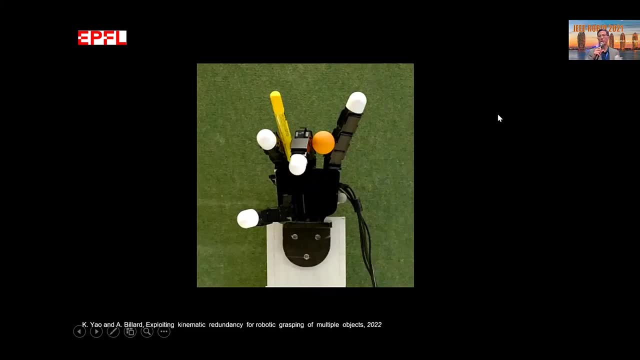 or you can just open your microphone and shout: Yeah, so can I ask a question? Yes, Yeah. So, Professor Bilat, thank you for your very interesting, inspiring talk. So I have been seeing that you had a work on the coordination of the dexterous hands, the fingers, 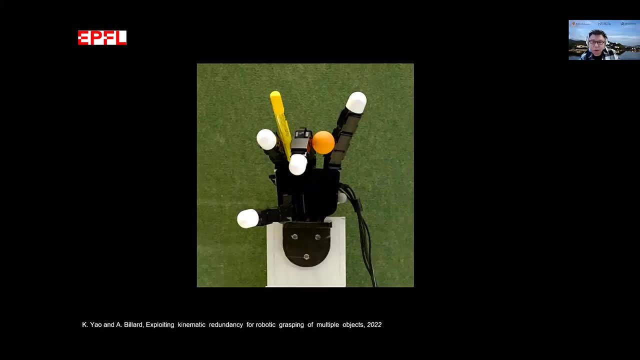 Also, I see you have some current work with the coordination with the bimanual arms. So my question is: how do you see in the future the coordination of the arm and hand And also, in particular, the bimanual arms and hands? 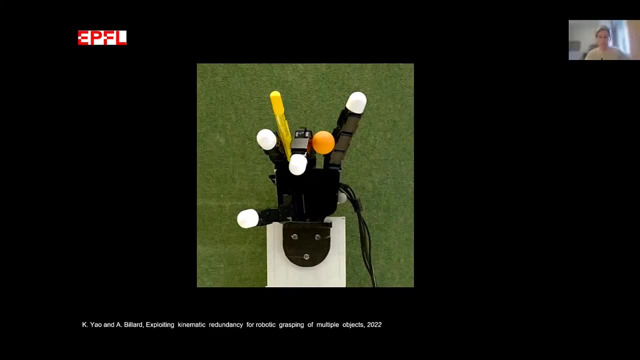 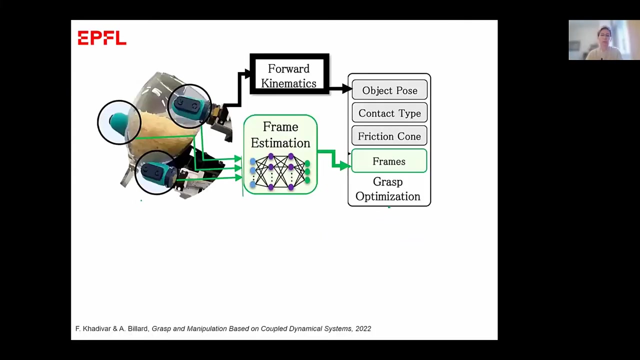 Yeah, Yes, thank you for the question. So we have also looked at that. I think it's extremely important. The way that we've proceeded was to. it's been shown very briefly through the just if I just go back to the handover video: 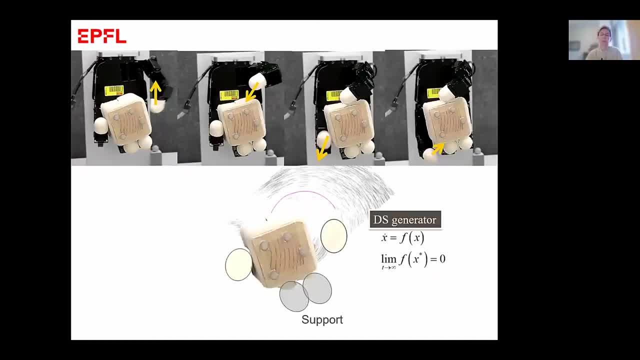 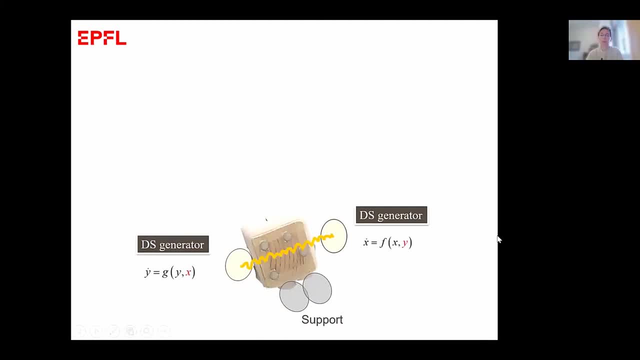 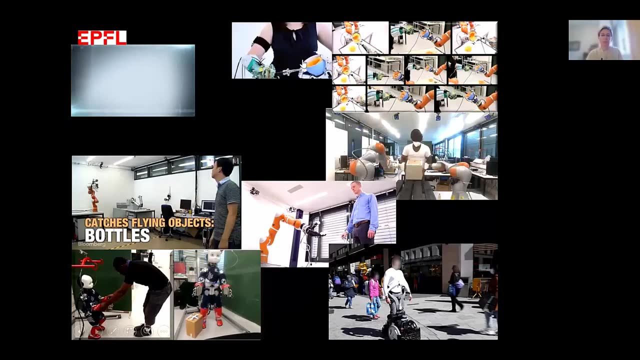 that I showed extremely briefly, at the very end. So what, we let me just. maybe I should share screen differently, because that's too slow this way, If you pay attention, I'm going to stop all those videos and just show you the one I'm catching up. 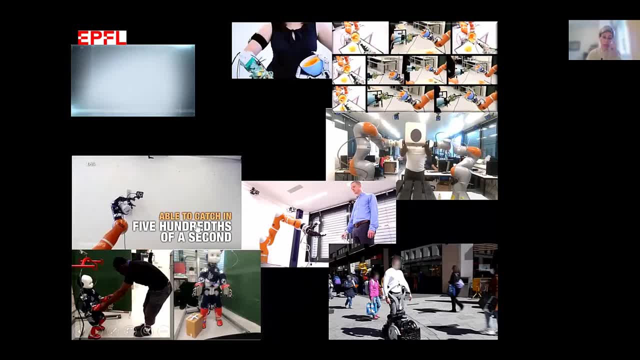 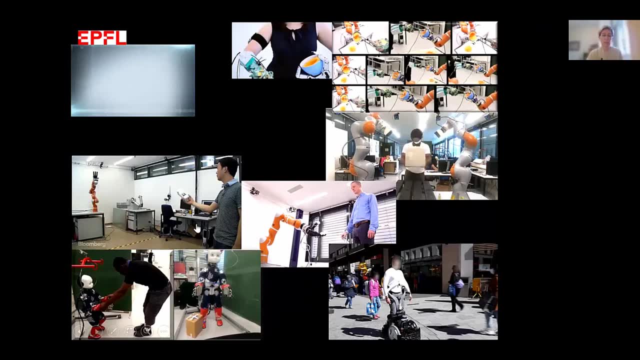 So for this one we looked extensively at the coordination. It's absolutely crucial. If you pick up and catch object like this, you need to coordinate the closure of your finger with the actual hand, The actual motion of the arm. So we have a temporal coordination. 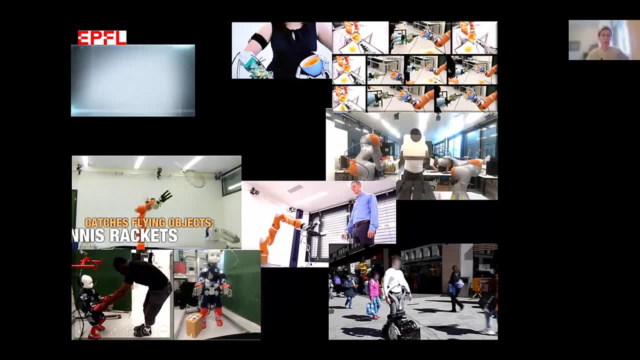 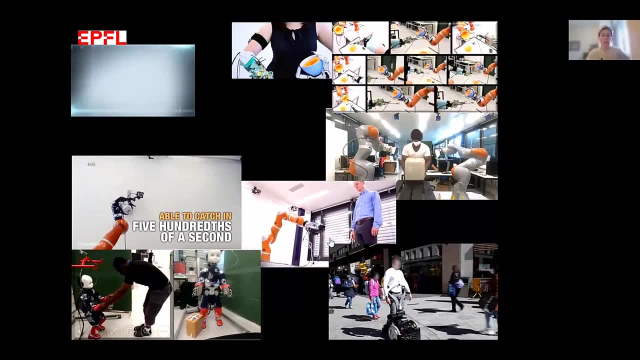 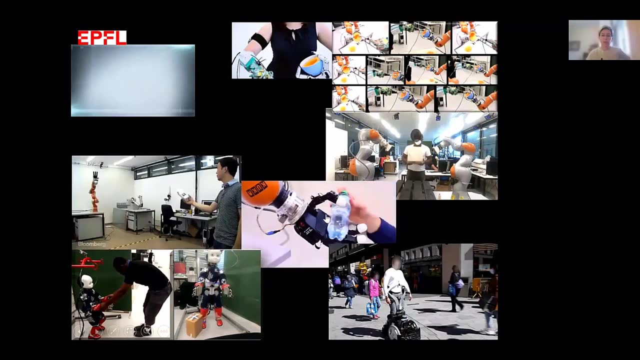 And this is similar when you pick up here from a human to the robot. Now there are differences in this coordination. Typically, here we have a sort of a leader follower type of coordination. If you observe this, you'll see that as soon as the object is put in the hands, 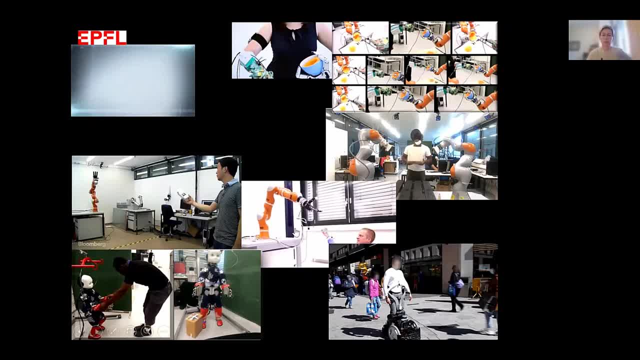 then the robot arm stops. That means that as soon as we perceive that we place an object and that there is force applied on the hands, then the hand closes, And as soon as the hand closes, then the arm stops, And so this coordination can be built. 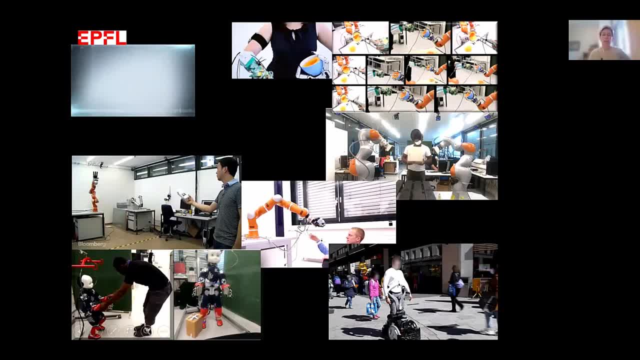 For this we use also dynamical system control And we use a coupling between the two with a codependency, but where the leading system is the hands and the dependent system is the arm. When you look at this other video, where the two arms are coordinated, 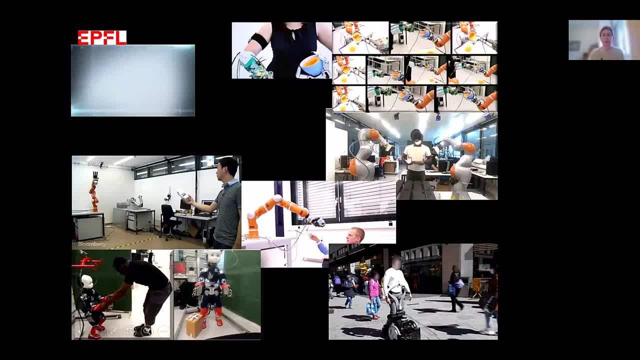 this is also a coupling. you have here A coupling between the two arms. They are here coupled to move in synchrony, similar to the finger coupling that I've shown before. Now, we have never done what you're suggesting, which is to couple now two hands. 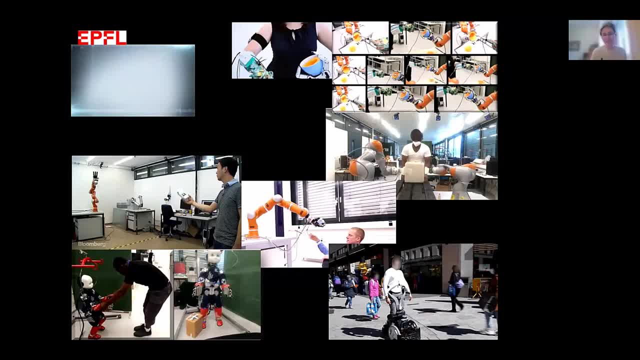 and all the fingers in the hands. with the two arms It would be possible. There is nothing that prevents it. We haven't taken the time. I don't think that there is any novelty to that, because it would be essentially putting together things that we've developed so far. 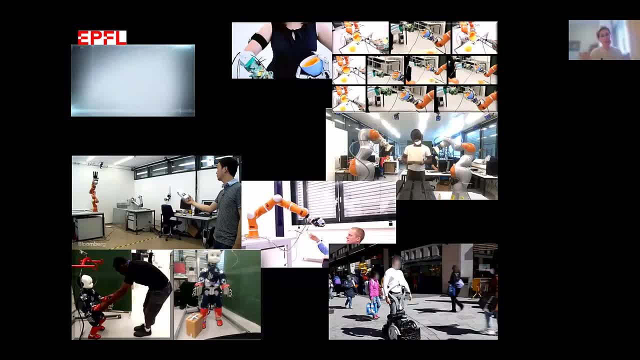 but it's totally feasible. Possibly what could be novel and interesting is if this co-adaptation had to work also in force and torque control, which I haven't touched upon so much. Clearly, we may have to think about how to rebalance. 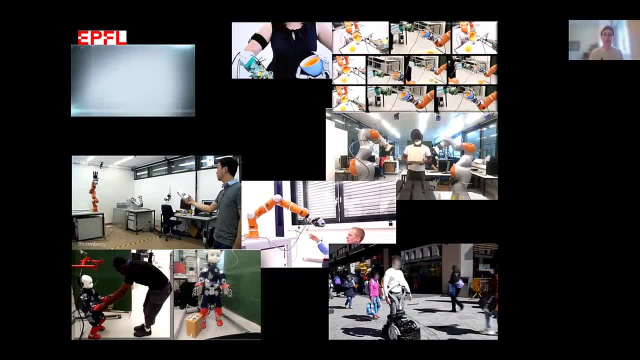 the forces across the two arms and possibly also changes the finger configuration in synchrony to this rebalancing of the force across the two arms. That is something that could be quite interesting, because that will call for possibly extending this notion of the feasible grasp on the workspace. 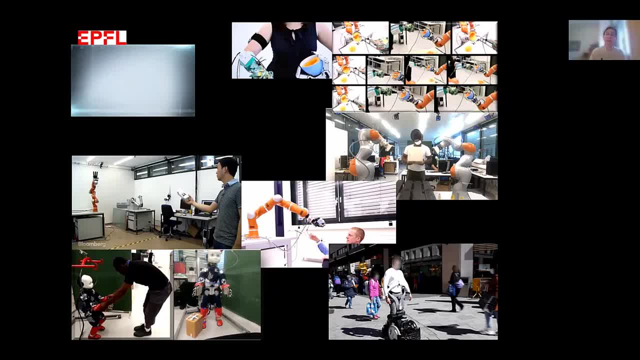 to the arm and hand, as opposed to just compute it now for the fingers, And also to take into account force. Yeah, sorry, Yeah, I'll stop here. Okay, thank you. Thank you, Great. Maybe it's the on-site audience turn. 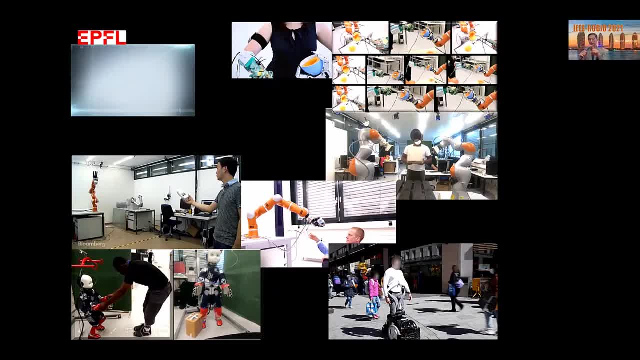 Anybody else? Yeah, we do have a few minutes, which is good. Yeah, we do have a few minutes, which is good. Hello, Hi, Can you hear me? Yes, I can hear you. So you were talking about biomimicry. 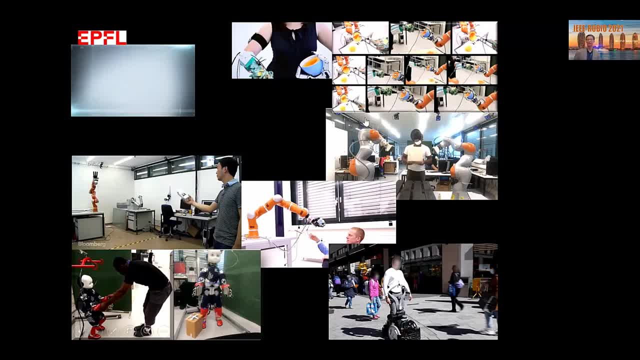 and also how anthropomorphic hands they might not be just completely replicated, in the same way that I mean the control methods that we have for humans should not be replicated for robots. What about the construction? just trying to emulate human hands by creating anthropomorphic robots? 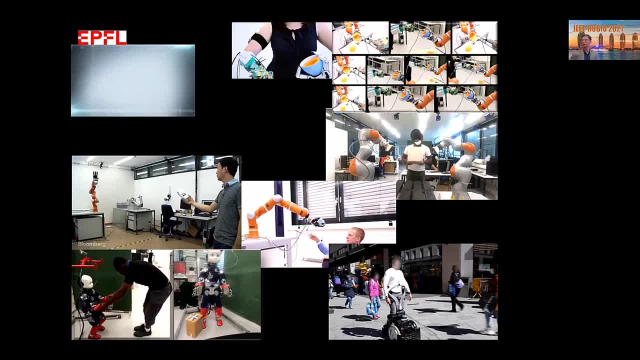 Do you think that in the future- let's say five, 10 years from now- we will still have robots still being created with anthropomorphic hands, Or do you think that maybe there is a design that will eventually transition out of anthropomorphic and have only two or three fingers? 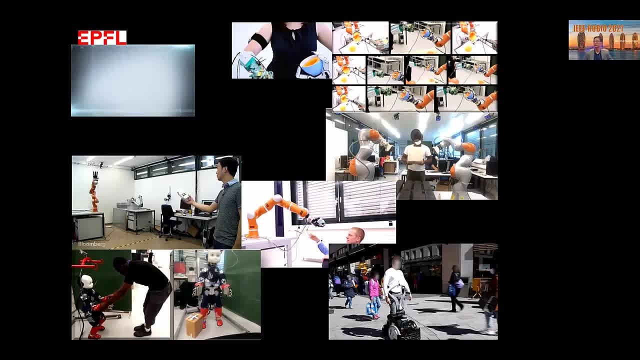 Yeah, thank you for the question. So you know, anthropomorphic hands make total sense when you want to design prosthesis. So in that sense I think there will still be quite a lot of work on that And so far prosthesis have only five degrees of freedom usually. 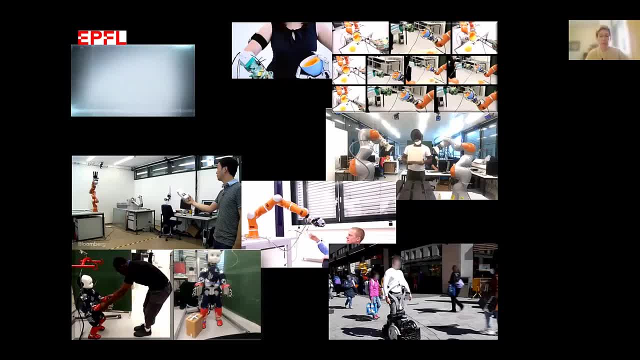 So, in comparison, when you think of the Allegro and the iCub hand that I've shown here, they have much more degrees of freedom, but they are much more flexible, And so you know there's a lot of work to be done on that. 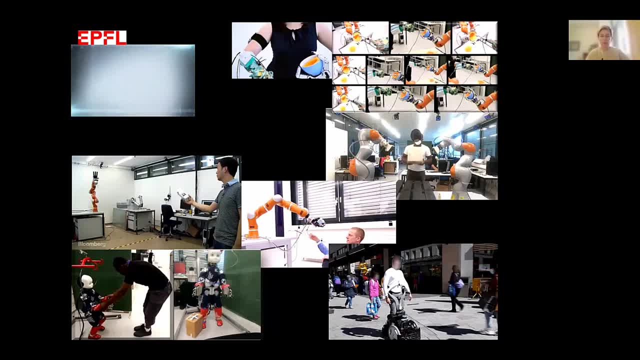 They are very bulky and heavy, So I believe that there will still be tremendous amount of work to be done on reducing the size and the weight of those dexterous anthropomorphic hands to use them as prosthesis. There are also advantages to use anthropomorphic hands. 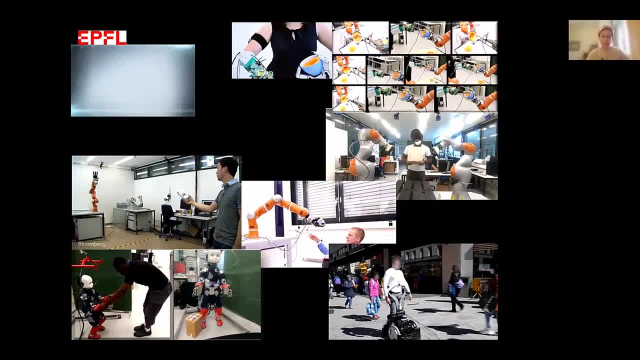 if you want a robot to interact and work with humans, because it's probably easier for the humans to predict what the robot will be doing, because it has this image of what the hand would look like. So that's one of the advantages of anthropomorphic hands. 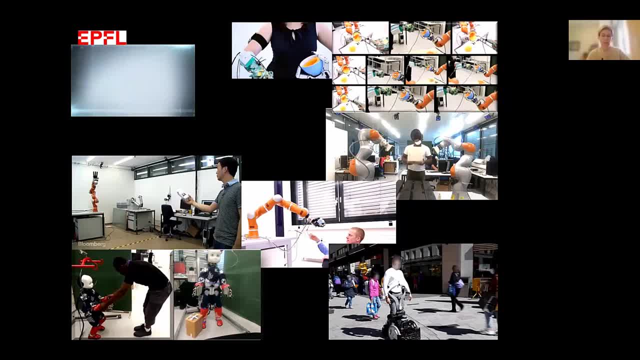 But when it comes down to pure robot control, yes, I would love to see people think about different types of hands, not just gripper, not just three fingers- You could actually put more fingers. What I would love to see- and I don't know if you see my video- 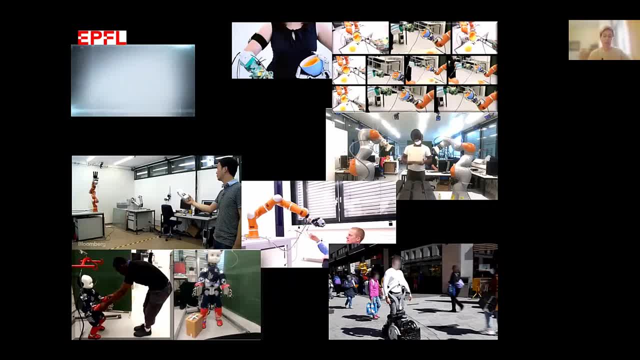 but I would love to see also hands that can pick up objects from front and below. I have also. I don't have them here, that's too bad, but I had a couple of drawings. These are things that I had someone make for me. 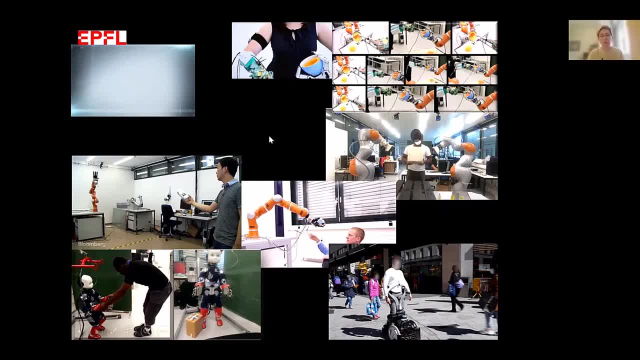 of a hand with two thumbs because the thumb is so dexterous. It's a wonderful kinematic. We have only one and it makes our hand very asymmetric and leaves us with the pinky and ring finger that barely do anything. Why don't we have two thumbs? 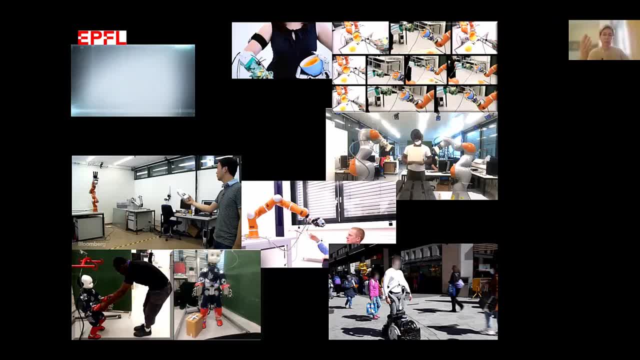 as opposed to one pinky and a thumb. That would increase enormously the dexterity and that's something that we see. if you are familiar with the work done by Etienne Bourdet, who studies the population of humans that have six fingers, 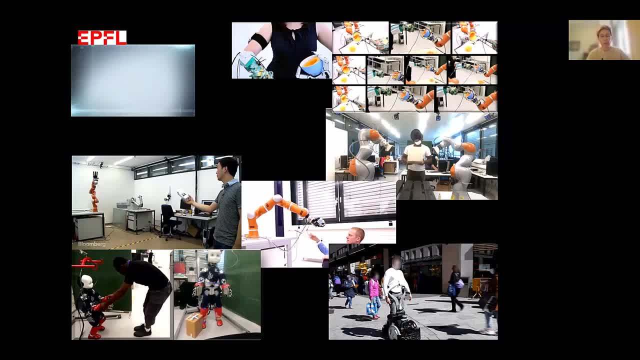 They are born with six fingers. Then they manage to use some of the fingers with the dexterity of the thumb and index and some of the pinky and the additional finger that they have. So, yes, we could think of having hands that are non-anthropomorphic. 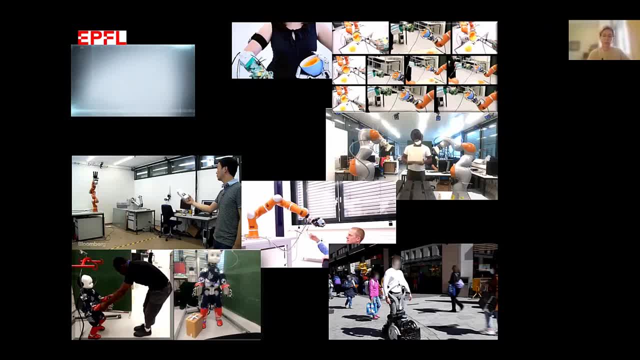 that have much more fingers or less fingers, especially also fingers that move different ways, And that doesn't you know, that doesn't apply just to hands. Think of robotic arms. They are all similar. You see one more company coming up. 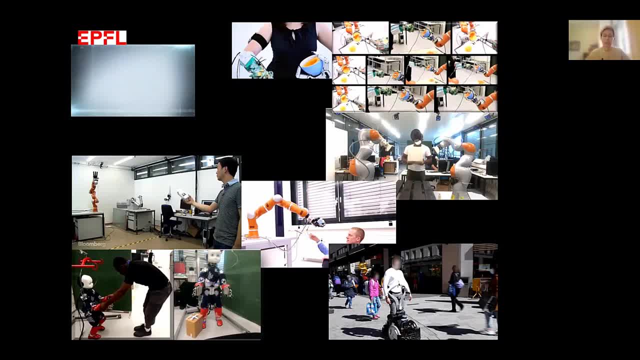 again another seven degrees of freedom arm, exactly the same as all the ones that we've seen before. We lack tremendously imagination in terms of mechanical design. So you know, I love the question. Thank you very much And I hope that we'll see more designs. 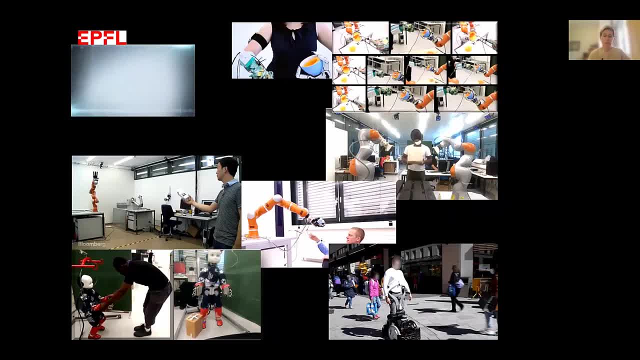 that are going beyond anthropomorphism for robotic purposes. Thank you very much. Okay, yeah, So maybe I can slip in a question myself. Yeah, so you haven't really touched too much on the perception side of the problem. I see you rely heavily on motion capture. 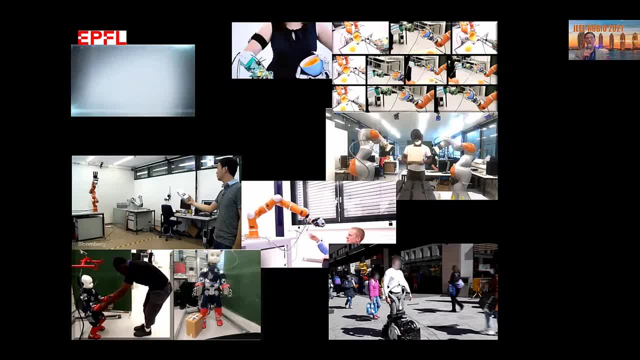 You have a bit of tactile sensing, So can you just comment quickly on the challenges that are facing the perception of dexterous manipulation? Yeah, thank you Zilong. So, but you know when you're doing hand manipulation. 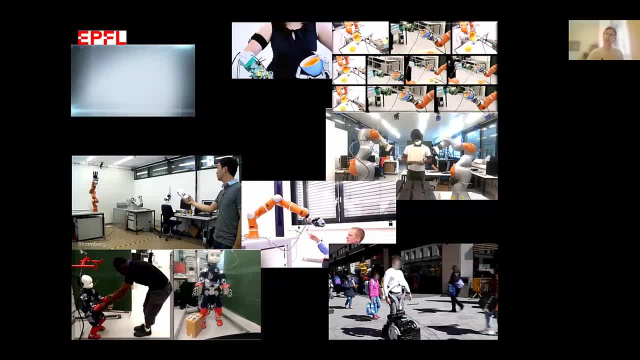 I believe that the perception you really care about is tactile sensor, is force touch sensor- And we do use them extensively- And whereas vision it's probably much less important, Because once you have the object in hand, basically it's obstructed. 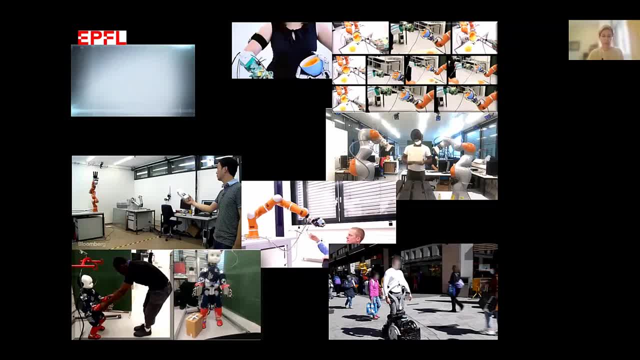 You know, you barely see it, especially when it's a tiny object. So vision is there, as it is for humans. It's there to allow you to identify the shape, to give you prior on the possibility of the shape, the weight and the texture. 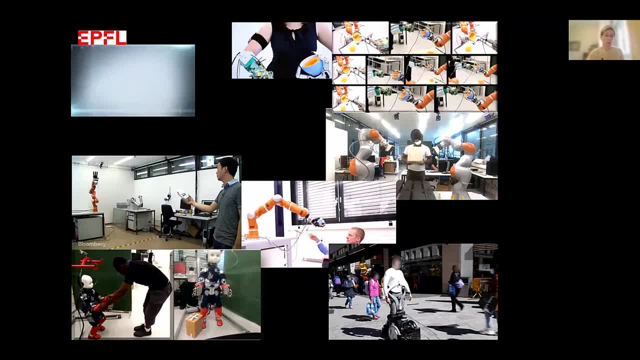 sort of friction coefficient. But once you pick the object, then you're left with adapting, especially when you pick it up and you move it in the air, And you have to adapt to what you're perceiving. So you could use vision also as a complement. 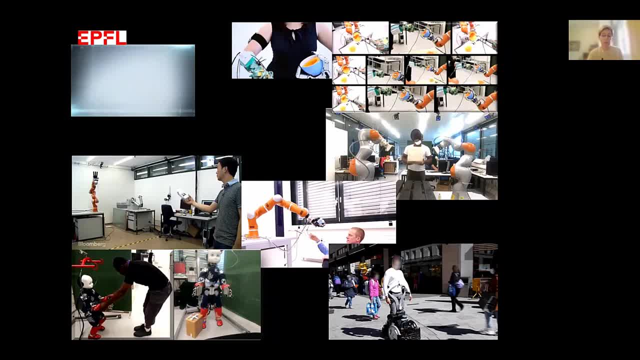 if vision was fast enough, That's true, and it would be very useful. And also if your vision was very robust to be able to pick up, you know, slippage, for instance, from seeing only partiality to have a partial view of the object. 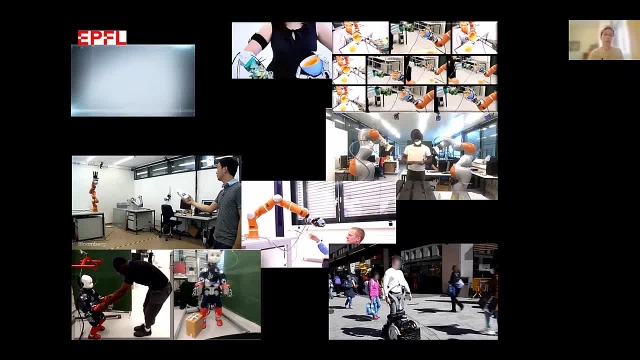 especially when it's a small object. So you need to be very quick at perceiving that to be able to separate the object from the hand. also, We're not computer vision experts, so that's the reason why we use OptiTrack Marker. 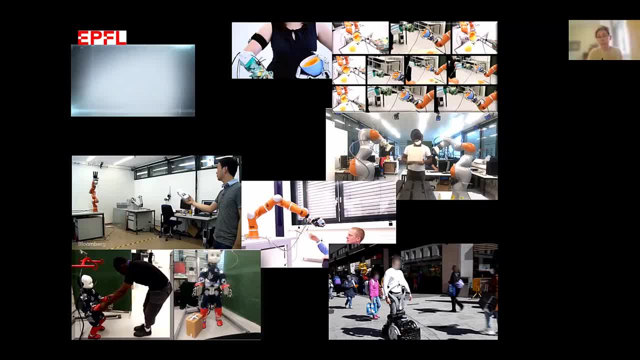 It's a field of its own, But whenever there is some state-of-the-art computer vision, we do use it. In truth, so far we found that it was very slow, Too slow for the type of in-hand manipulation, so that's the reason why we haven't used it so much in this work. 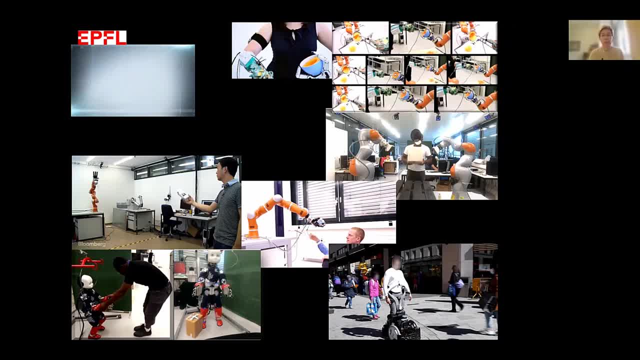 But if there were people interested in collaborating with us on this, I definitely would be extremely interested in that. Okay, so maybe one more question, either from audience here or online. Could I have a very short question? Go ahead, This is Zhidong. 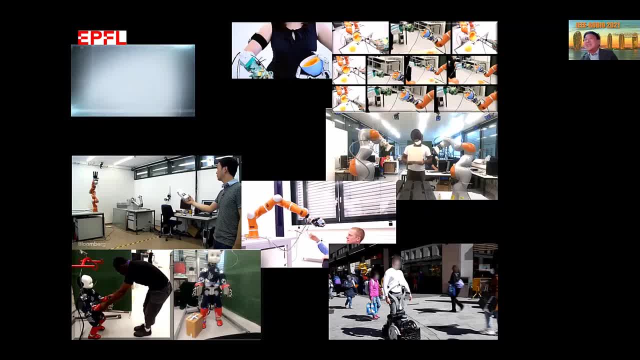 I'm really interested in how to do in-hand manipulation to spare human beings' skill. So you mentioned that they have a lot of grasping pose. So how do you commence the robotic skill, Different or similar with the human beings' grasping? 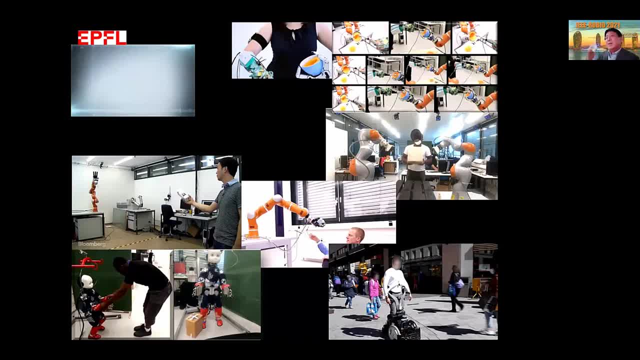 It was by chance, You know, in fact. so, at the very beginning, when I showed this similar grasp between the human hand and the human hand, this was not by design but because, if you want, it was not by design in the objective function. 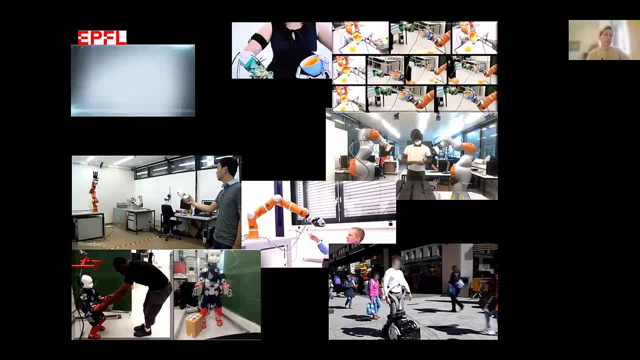 and the constraint-based optimization controller. but it's unsurprising because the hand of the iCub is very similar to the human hand. It's similar both in size as well as the placement of the finger, especially for the thumb, which is quite close to the motion of the human thumb. 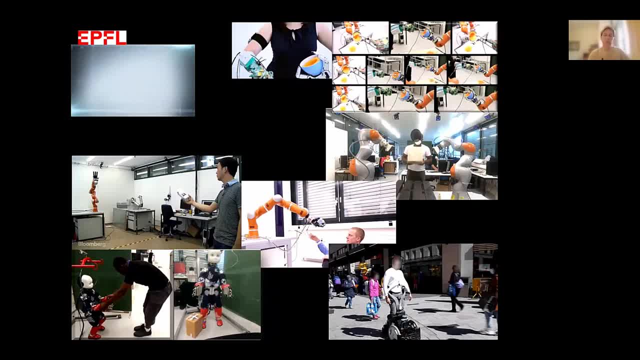 and for all the objects. So it's quite unsurprising that we end up with a set of feasible grasps that resemble very much the human one. I did not show that here, but we did the exact same optimization process for a three-finger, typical robotic hand. 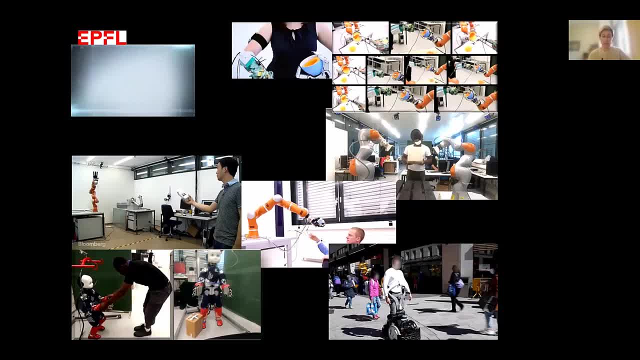 This was the Barrett hand, which has the opposing finger. I cannot really do it with my hands, but you have really fingers that can move around a circle with 360 degrees rotation. well, 180 actually for each of them and they can really have. 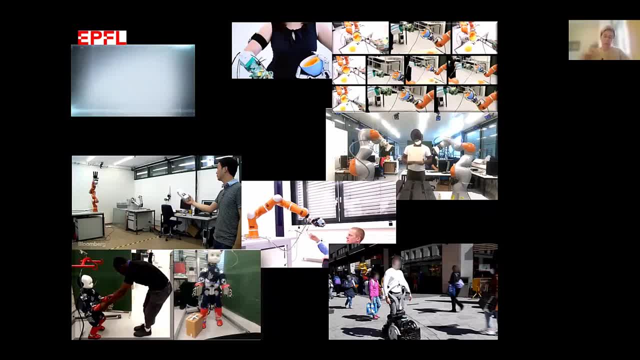 a completely symmetric distribution with the three fingers around a circle, And there you end up also with lots of feasible, interesting, amusing grasps. but they bear no relationship whatsoever to the human hand's type of grasp, So that depends very much on the kinematic of the hand. 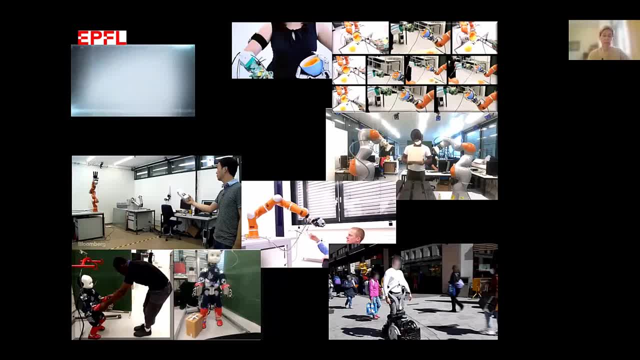 Similar kinematic will lead to similar feasible posture. Dissimilar kinematic will lead to other type, but still a range of them, other type of feasible posture on the object. So I hope it answers your question. Okay, So with that I think we are out of time. 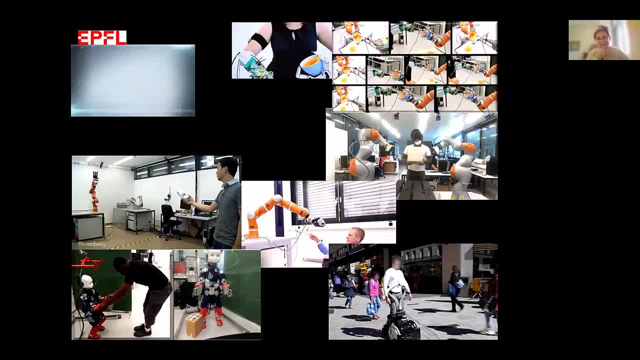 So please join me in thanking Professor Billard for a very insightful and entertaining talk. So thank you very much.